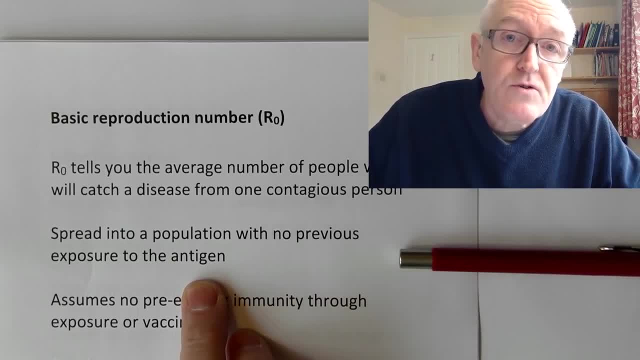 exposed And, of course, if you haven't been previously exposed, you haven't developed any antibodies. you've no immunity. that means you are very vulnerable to the disease. To you it is a new disease, You haven't experienced it before. And the thing about this antibody antigen thing- 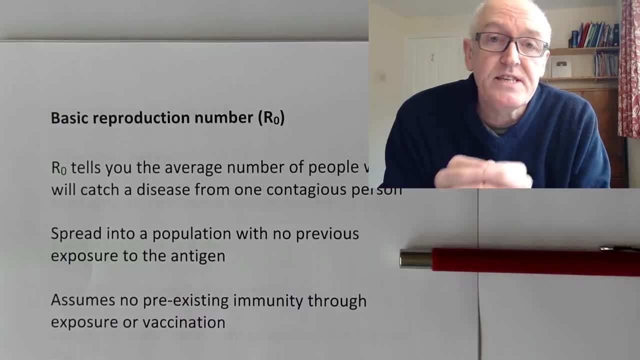 the antigen stimulating the production of antibodies. they are specific to a particular virus. So if you are immune to one bacteria, that's not going to make you immune to another bacterial illness, Or if you're immune to one virus, that's not going to. 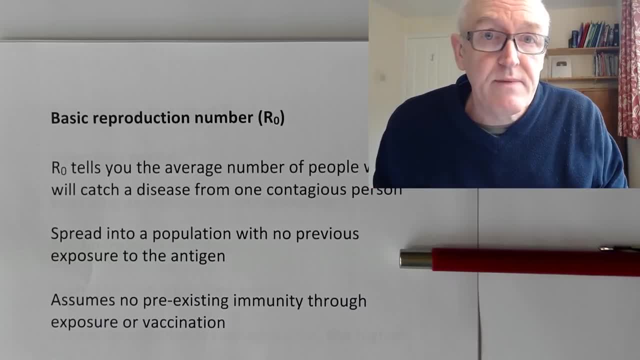 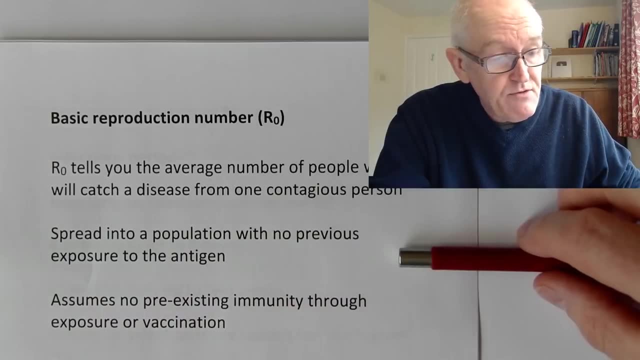 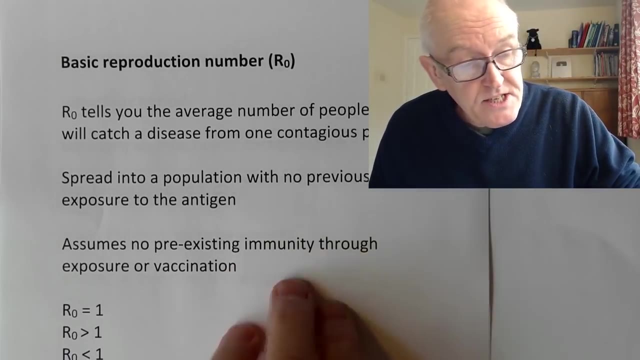 necessarily make you immune to another virus. In fact, it's very unlikely to make you immune to another virus. So this has to be done on a specific basis. So that's what the antigen antibody reaction is. We're assuming that people have not been exposed to the antigen, So, assuming no pre-existing 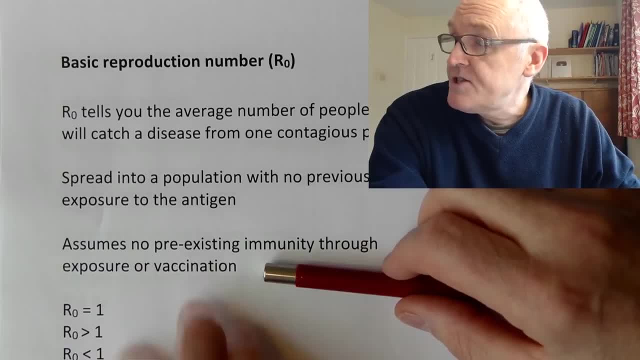 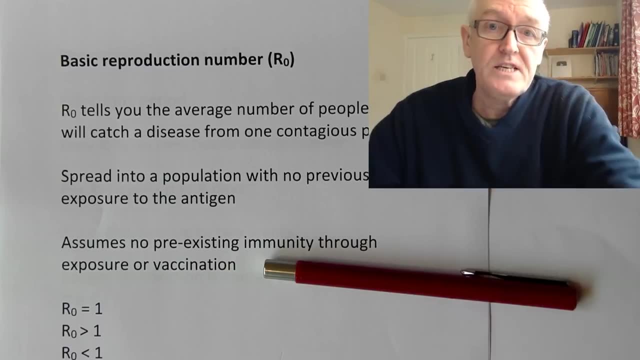 immunity through exposure, And this reminds us of the two ways that we can get these antibodies, that we can get this acquired specific immunity. One way is by suffering the infection with varying degrees of clinical manifestation, Or the other is that we're vaccinated against it, And this is the whole point of vaccination. 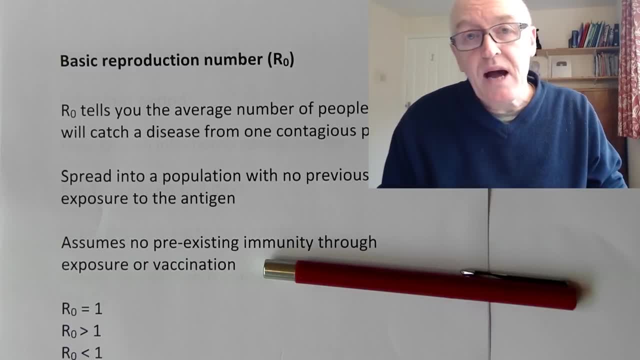 that we get the antibodies, we get the immunity, but without having suffered the disease, Because the vaccine is something which fools the body into thinking it is the disease Make. well, it can be parts of the disease. It's attenuated versions of the disease that won't make us sick. 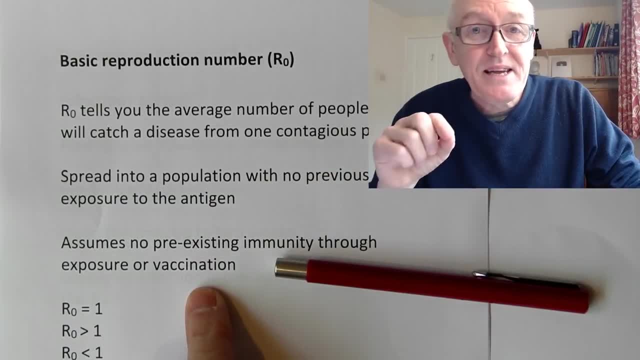 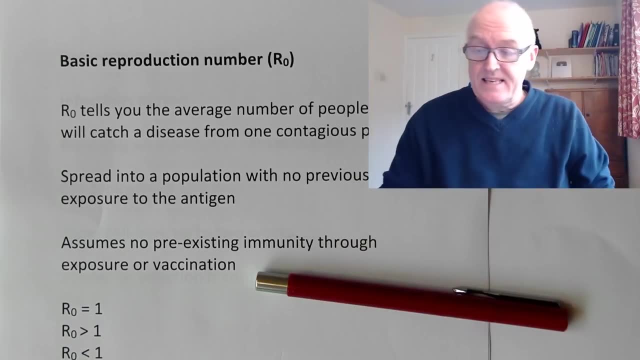 hopefully, And this stimulates the body into making antibodies, And then when the real virus or bacteria comes along, the body recognises it because it's been vaccinated. So just before we look at these numbers here, let's just look at what we mean by this in a practical example. 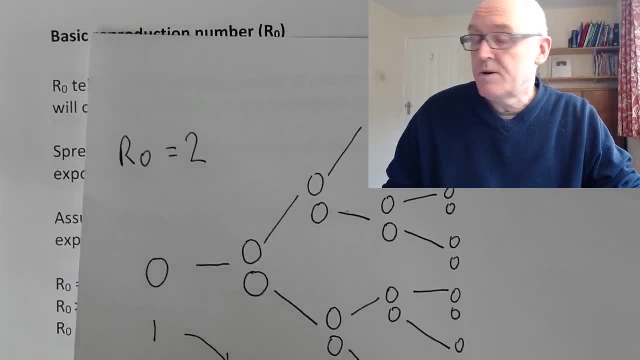 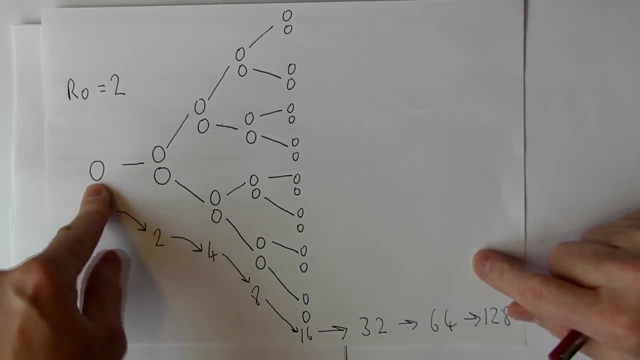 So if the R0 of an infection is 2. So in this example we see an R0 of 2.. So we start off with one infected person And that one infected person on average infects two more people. Then that infected person on average. 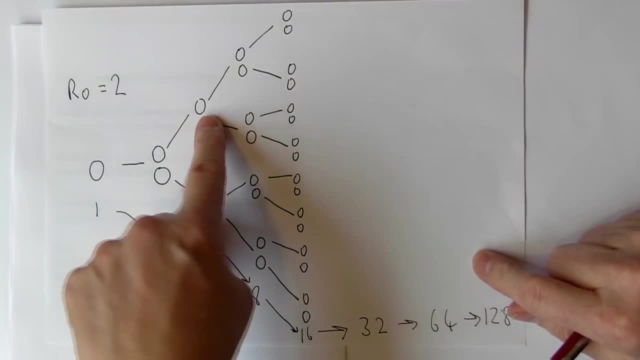 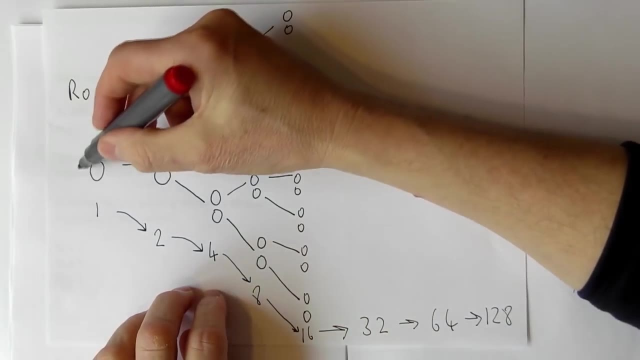 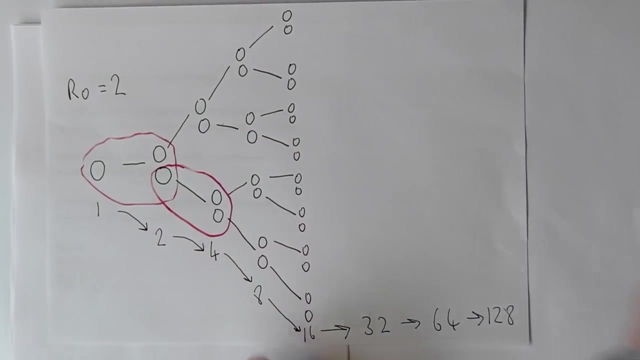 infects two more people, Then that infected person on average affects two more people. So we can see it's twos all the ways here. So one person here infecting two And then one person there infecting two And then one person there infecting two. 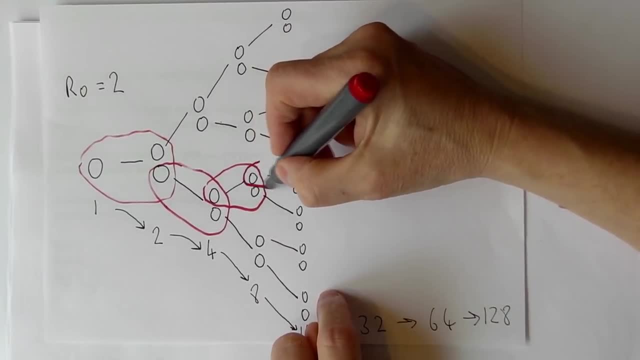 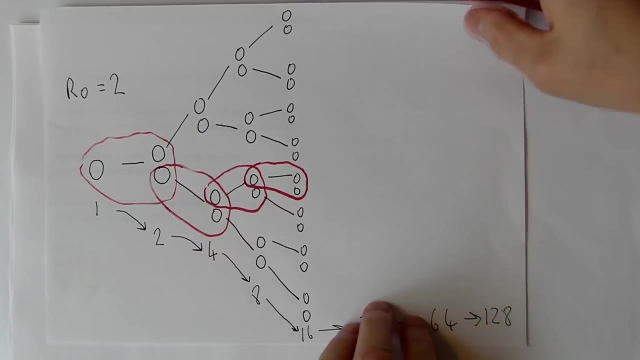 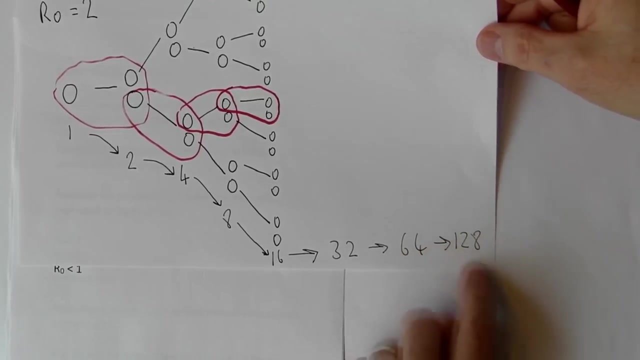 and then one person there infecting 2.. So the R0 is 2 in this case, But this means, of course, that we're going from 1 to 2 to 4, to 8, to 16, to 32, to 64 to 1 to 8 infected cases. 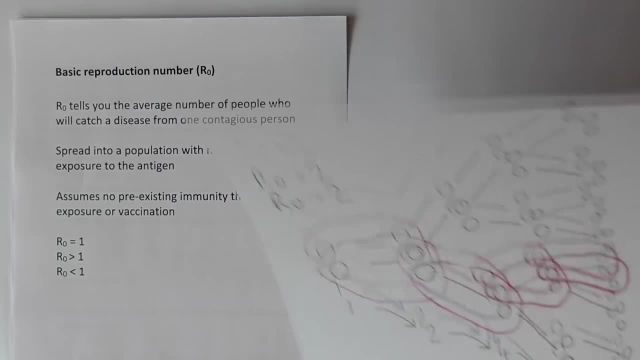 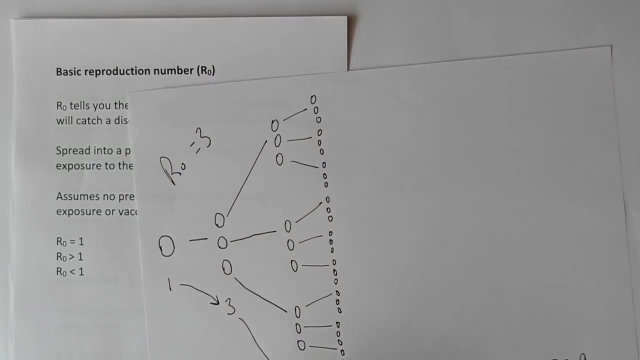 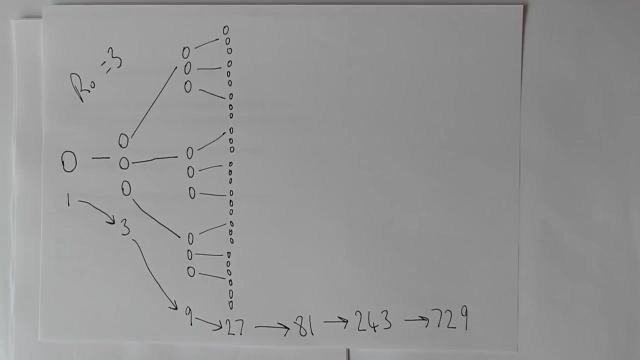 So that's if an R0 is 2.. Now if the R0 is 3, so in this example R0 equals 3.. So on average, 3 people are going to be infected per infected person. So here we have one infected person infecting 3 new people. 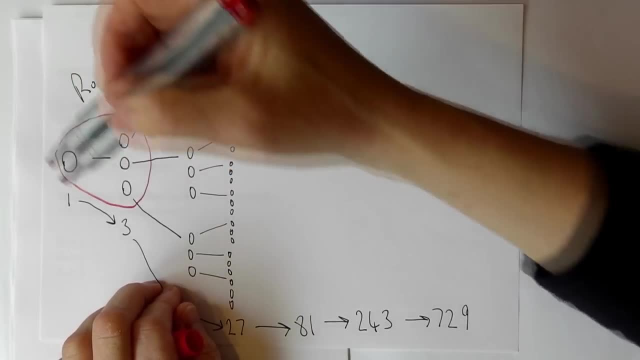 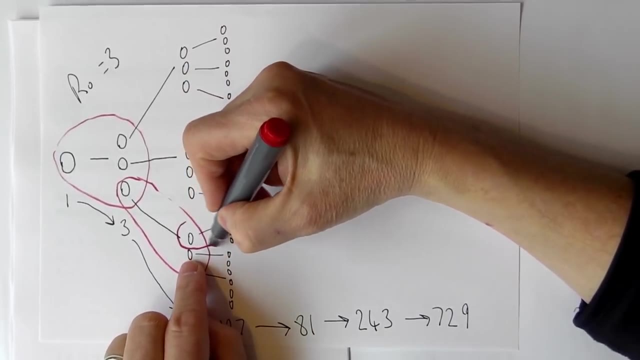 So that one person there is infected 3.. And then that one there is infected 3. And then that one there is infected 3. And that's the way it goes. Or we could take it up here That one person there is infected 3.. 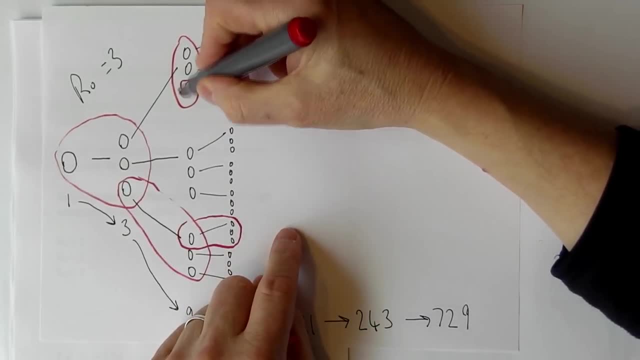 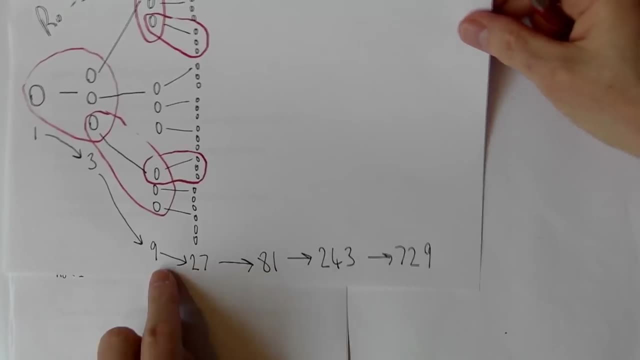 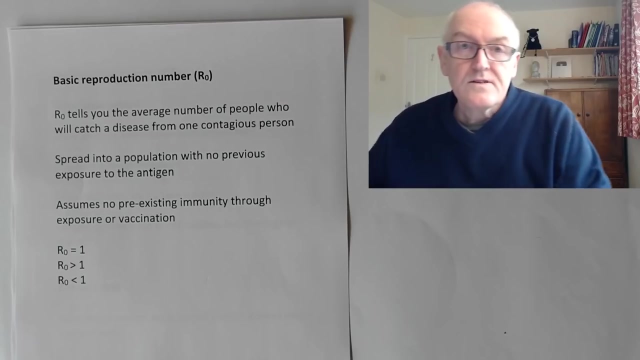 And that one person there is infected 3. Like that. So here the numbers, of course, of growth are much greater: 9, 27,, 81,, 243, 729.. Much greater rate of increase here. So we see this R0 value is absolutely critical to understanding. 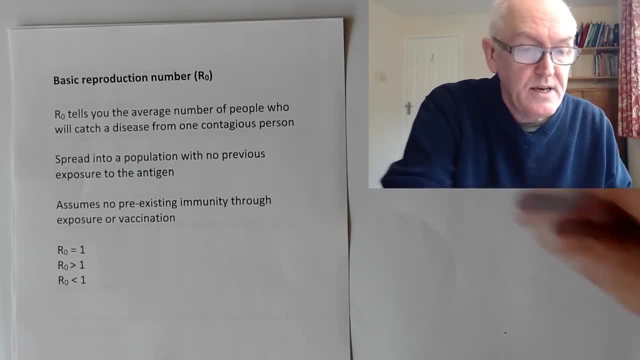 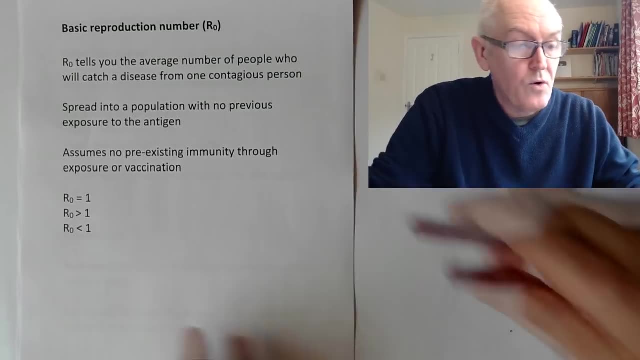 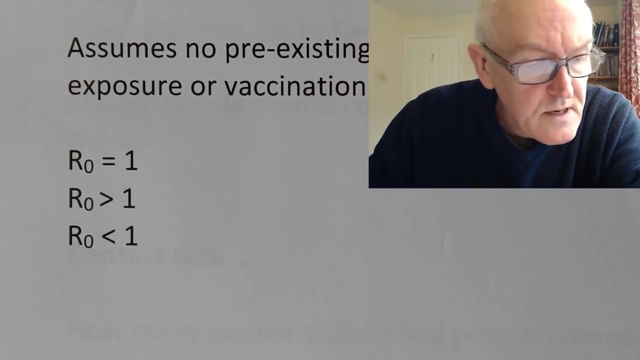 how quickly a disease can spread through a population and how many people can infect other people, And this is a very important concept Here. this R0, 1, whether the R0 is greater than or less than 1.. So just to focus in on this, if R0 equals 1,, 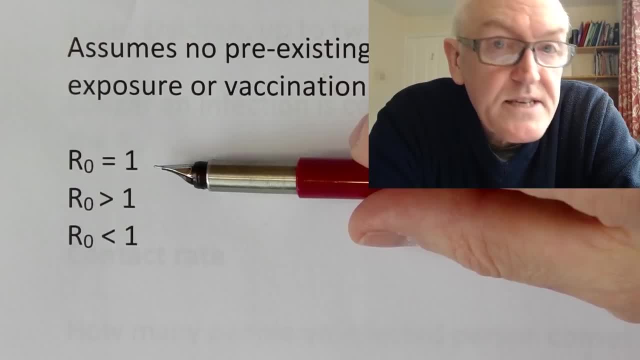 then that means each infected person is infecting one other person, So one person infects one person And then hopefully the person who was initially infected, who infected the second person, gets better. Of course they could die, But basically what that means is the one infected person. 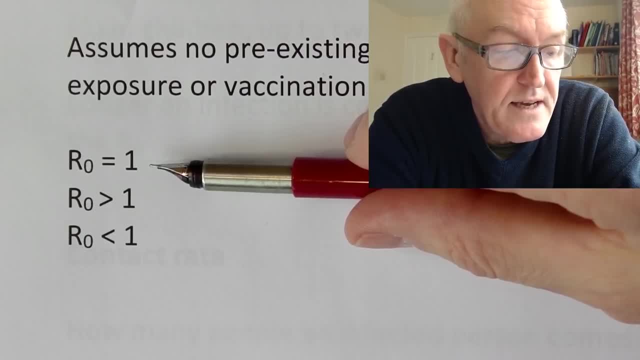 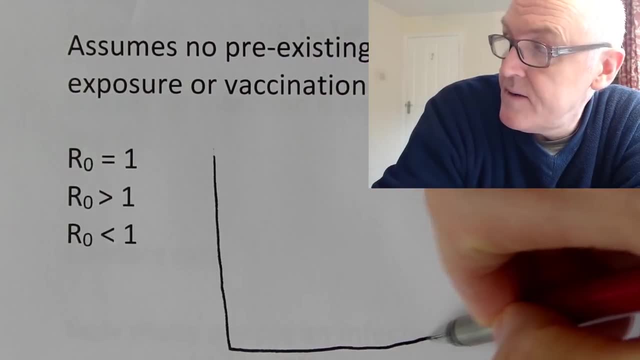 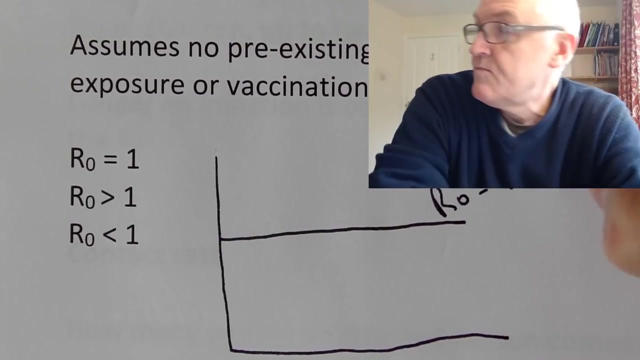 is replacing themselves with one other infected person. So that means the number of cases- if R0 equals 1, is going to stay constant. So that would be R0 equals 1.. The number of cases are staying constant in this case. 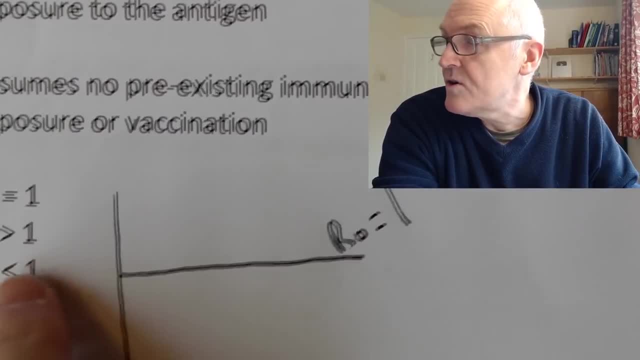 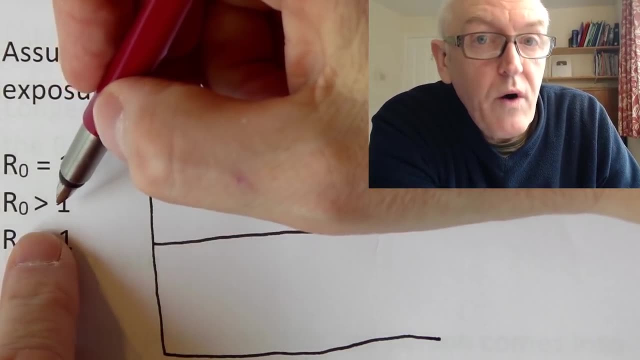 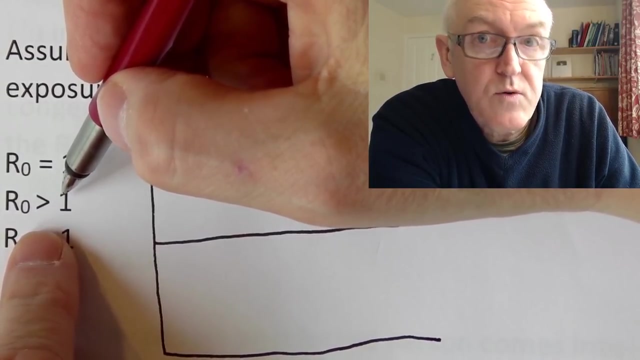 They're not increasing. Now, if the R0 is greater than or less than 1,, then that means that each infected person is infecting more than one other person, And the R0 could be 1.1, or it could be 1.2,, or it could be 5, or it could be 12.. 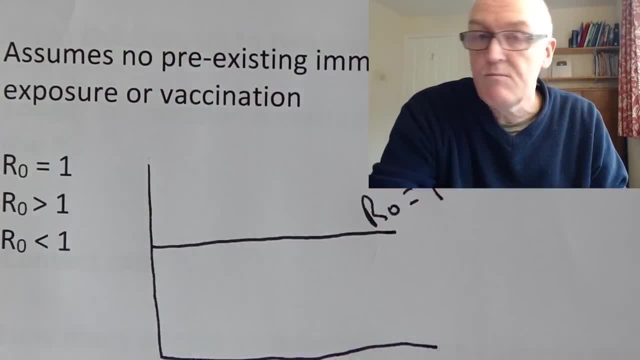 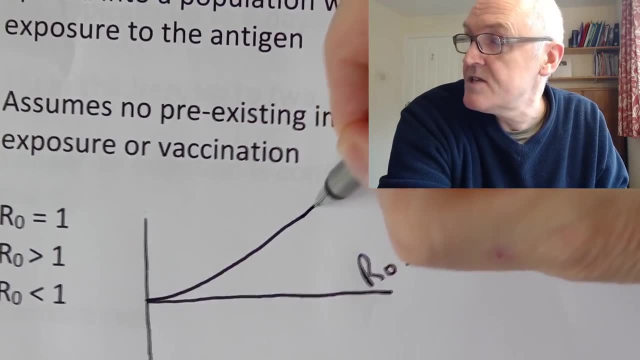 All of these situations, each infected person is infecting more than one other person And that means the number of cases will rise. So the number of cases will increase. So that line would then There would be: R0 is greater than 1.. 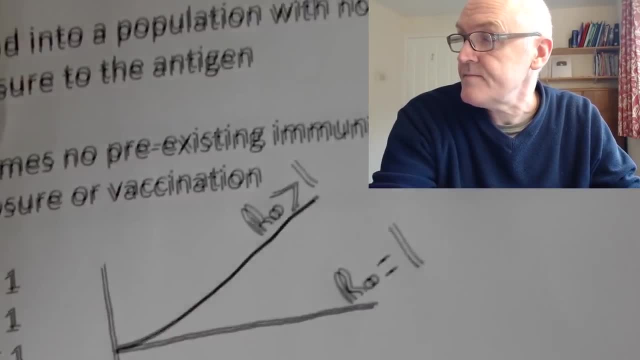 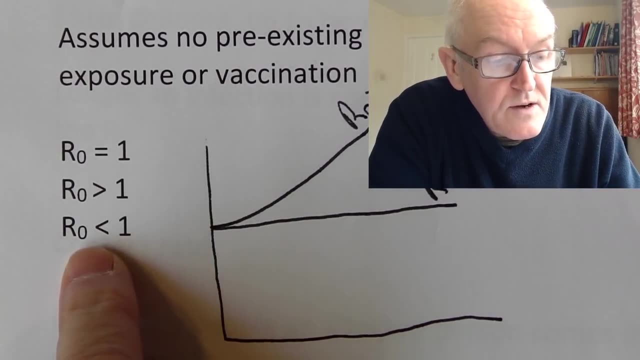 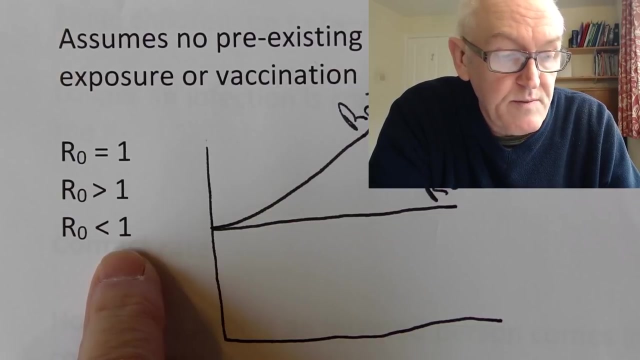 The number of cases will increase. But what we need to do in infections to stop the spread is to get the R0 below 1.. So if the R0 is below 1, that means on average each infected person will be infecting less than one other person. 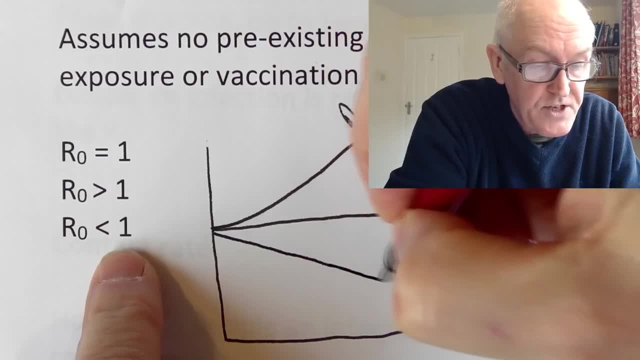 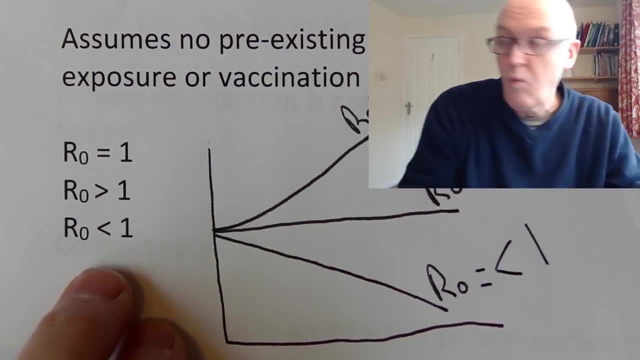 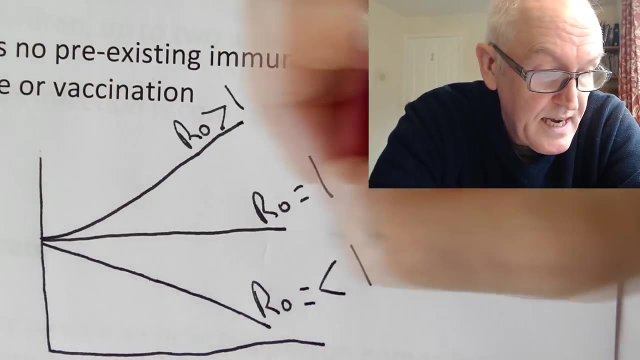 So that means the number of cases are going to go down and hopefully eventually the disease will disappear. So that line, there would be R0.. R0 equals less than 1.. So they're the three possibilities. really, R0 is 1, in which case everything will stay as it is. 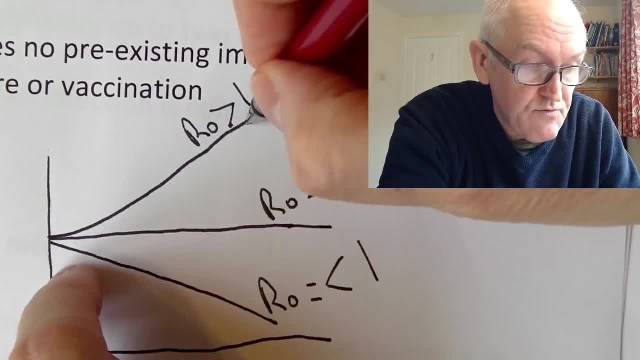 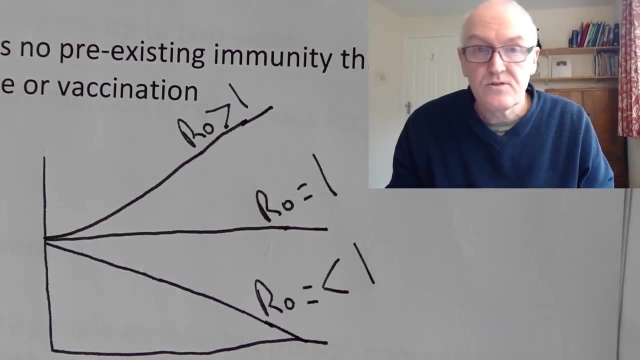 R0 is greater than 1, in which case the numbers of cases will rise. R0 is less than 1, in which case the number of cases will fall and hopefully eventually go down to zero. Now, what are the factors that determine R0?? 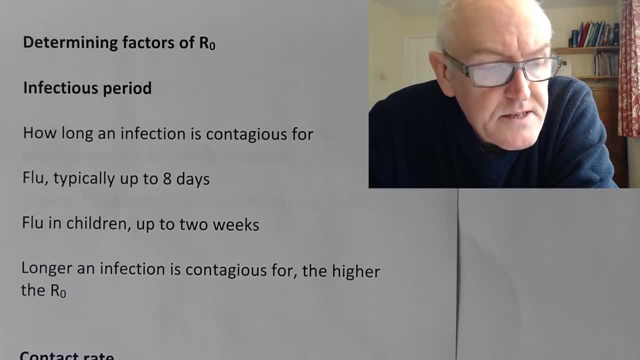 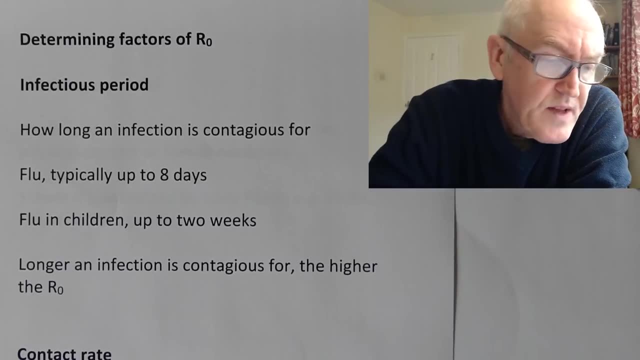 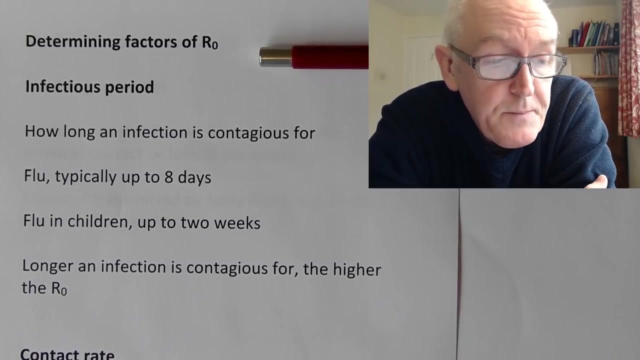 Well, R0 is determined by several factors, And some of these factors are biological And others of these factors are non-biological. So the R0 is not an intrinsic property of an infectious disease, of a virus or a bacteria. It depends on partly the biology of the virus or bacterium. of course, 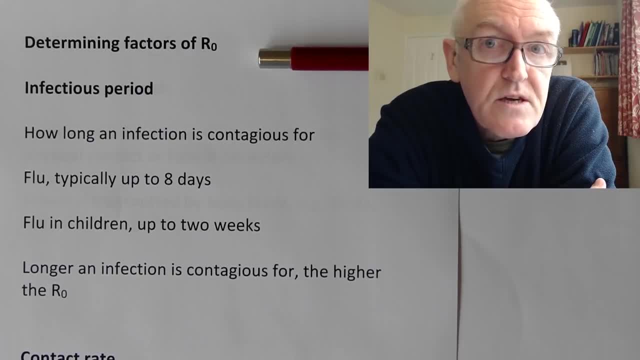 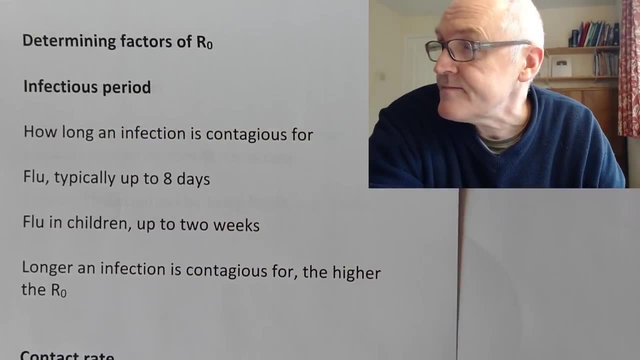 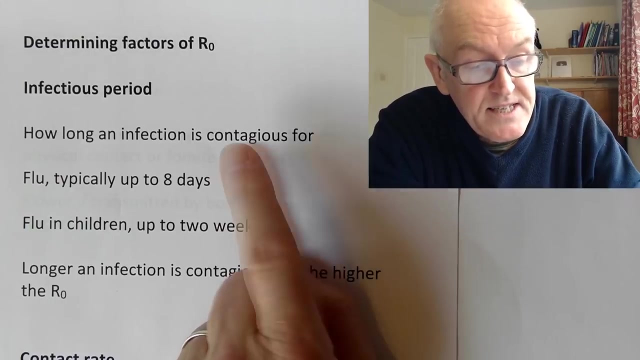 but also on how many people an infected person comes into contact with. So one determination, one determinant is the infectious period, And this is how long an infection is contagious, for How long someone can potentially spread. Contagious means someone can potentially spread the disease to others. 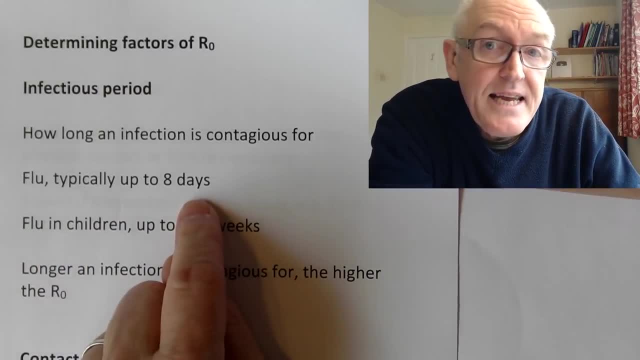 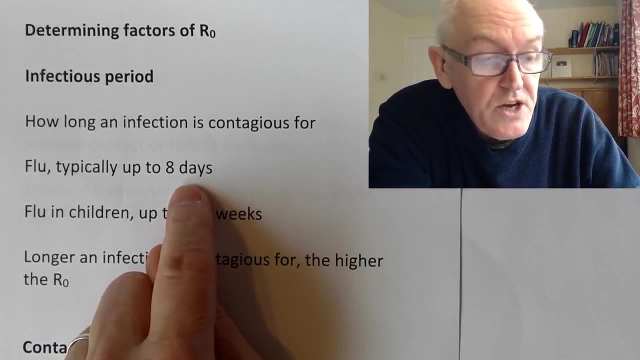 So for seasonal flu, for example, this is typically up to eight days. So with seasonal flu, someone is going to be contagious, able to spread the disease to others, usually for a day or two before they get the features, before they get the clinical features. And for some days after they get the clinical features. In children it can take longer, up to two weeks, probably because in children they haven't been previously exposed to similar viral flu infections, influenza infections, and it takes them longer to mount a full immunological response because the 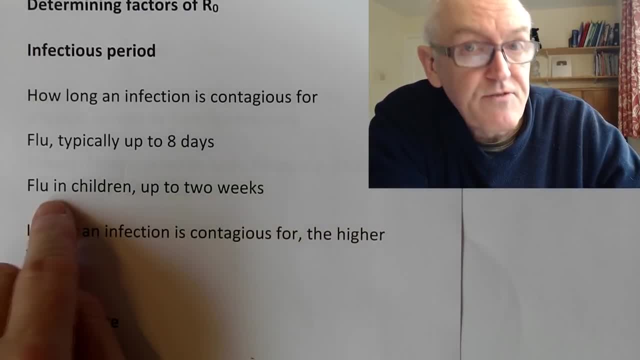 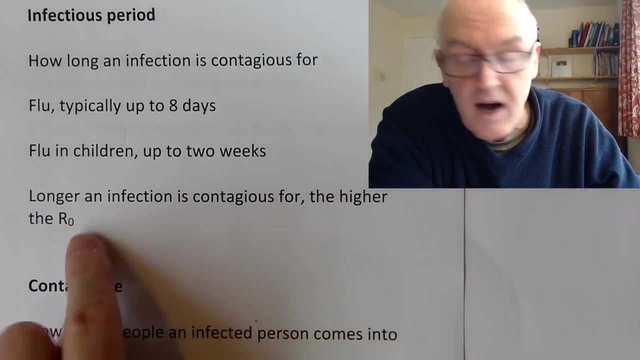 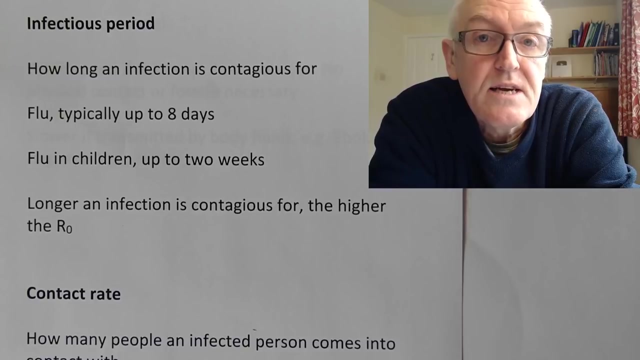 immune system has no previous training to this particular flu or influenza antigen. And the longer an infection is contagious for, the higher the R-naught. So length of contagion during any particular condition is going to tend to increase the R-naught. So that's really a biological factor. 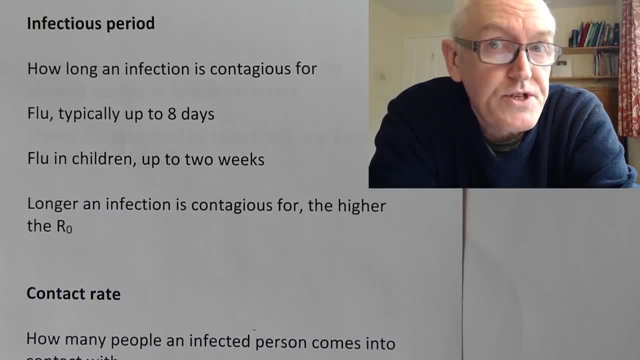 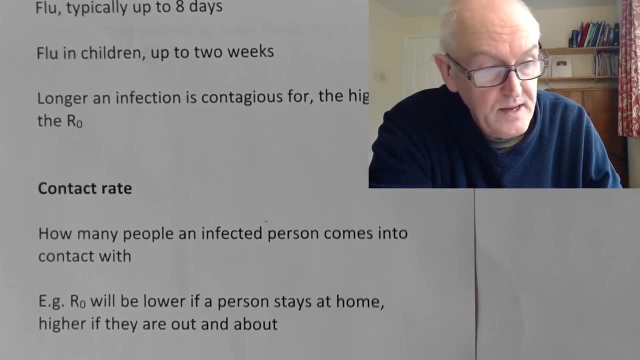 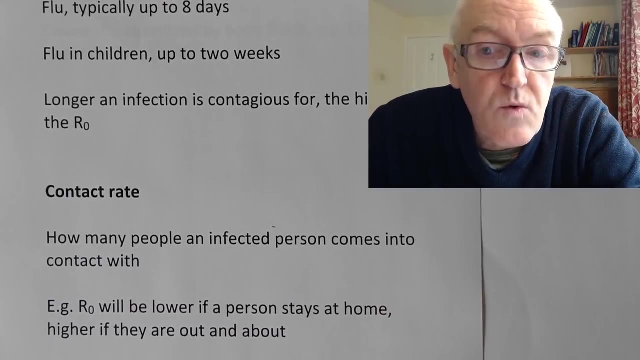 That's due to an interaction between the infection and the host, the host being the person that suffers from the disease. Now, contagion rate: how many people an infected person comes into contact with. So we have a person with the most infectious disease in the world. 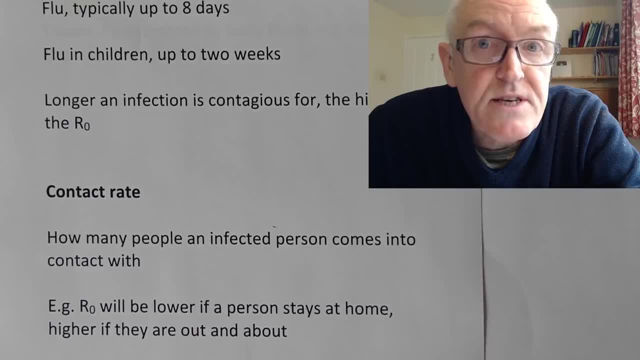 but the if they're isolated on a Pacific island, then they're unlikely to spread it to other people, because they're not coming into contact with other people, because by their very nature these diseases are transmissible: They must be passed from one person to another. 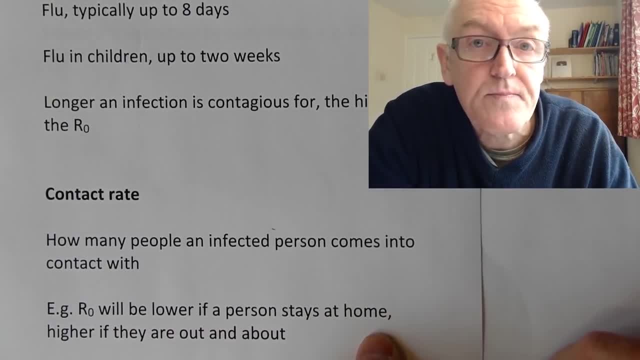 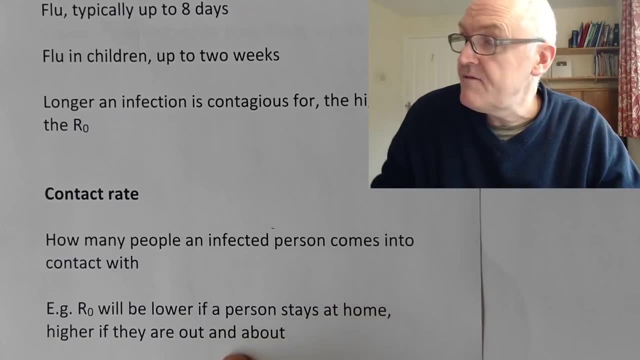 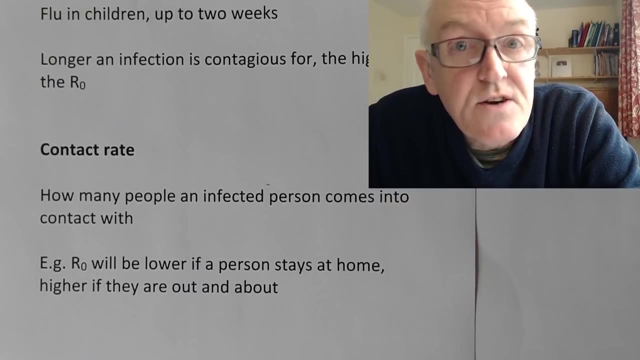 So the R-naught will be lower if a person stays at home and isolates themselves or if they live in a remote location, whereas the R-naught will be higher if they have more interactions with other people, more interactions. the nature of those interactions will depend on how. 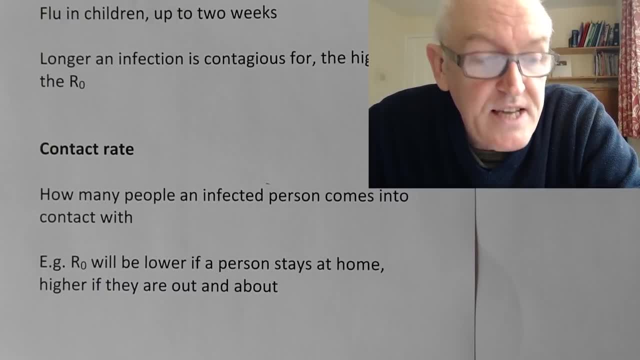 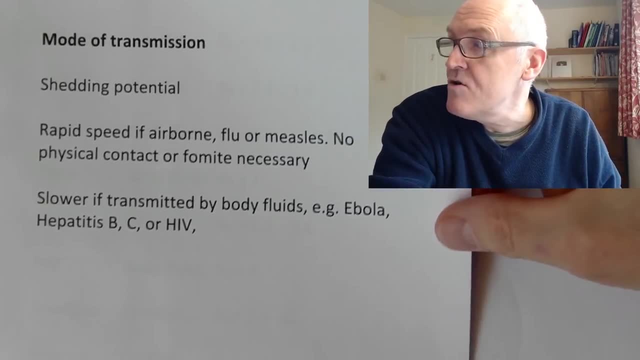 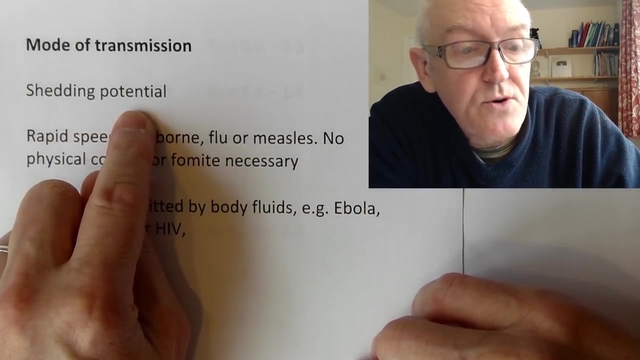 the infection is spread, But the more interactions they have with other people, the higher the R-naught will be. Another factor is the mode of transmission, And this is important because this influences the shedding potential of the virus or the bacteria. Now, the shedding potential is. 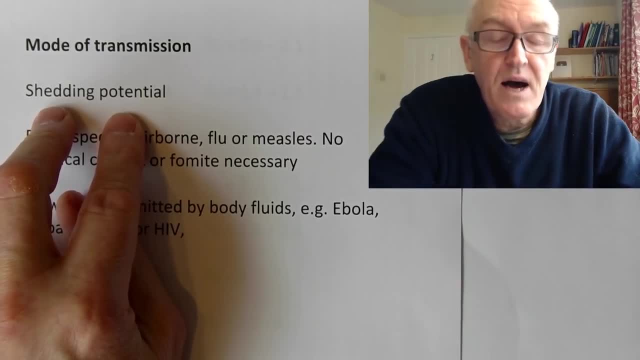 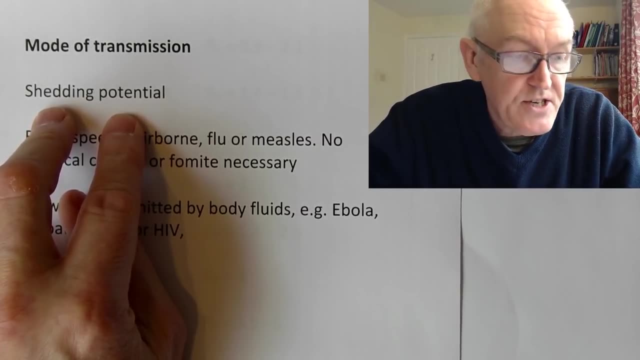 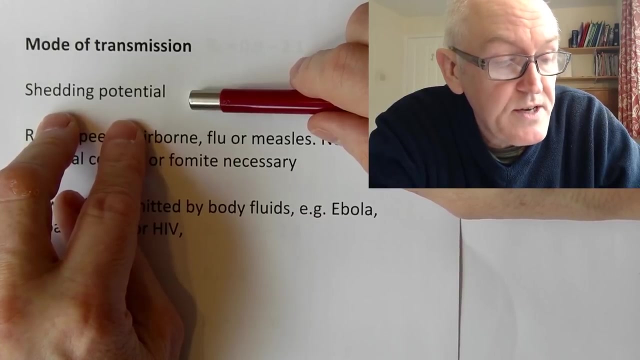 if I'm an infected person, how many viruses or bacteria am I giving out into the infection environment through my breath or through my body fluids or whatever it is? how infectious am I? what's my shedding potential? so this is important. so, for example, with HIV, human immunodeficiency virus, 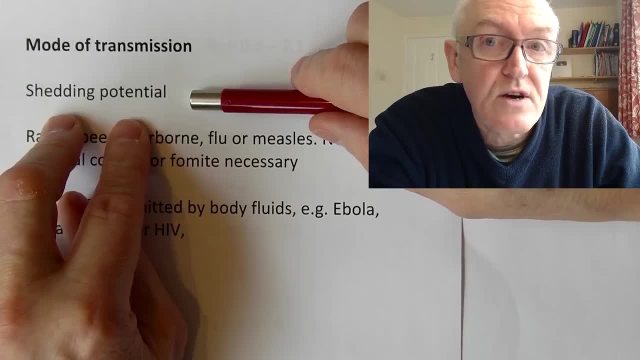 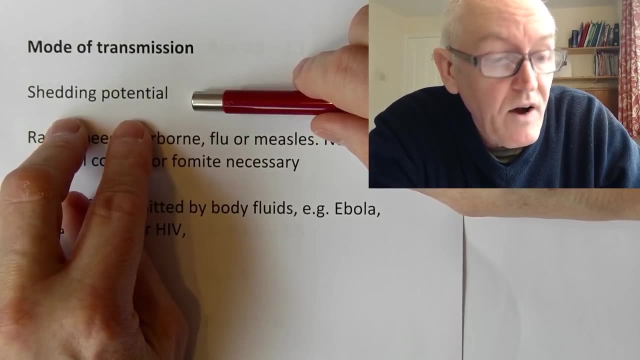 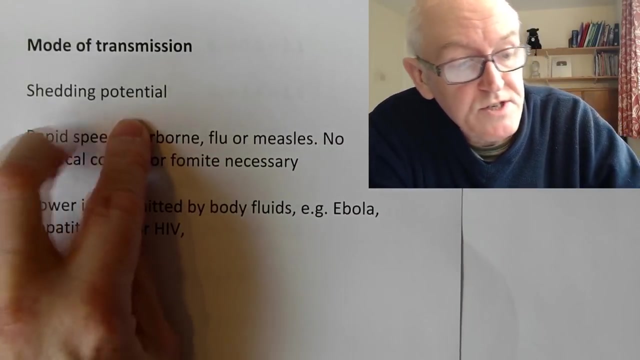 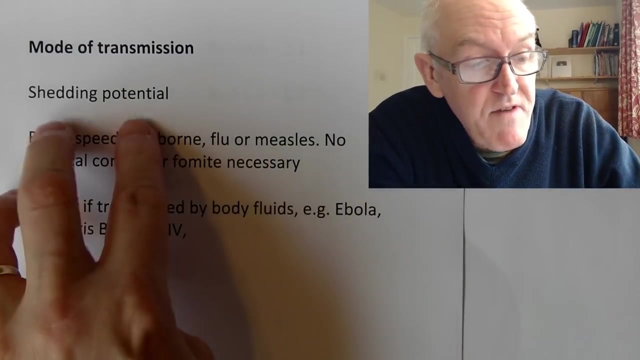 the shedding potential is reduced with antiretroviral drugs that prevent the multiplication of the virus, the RNA virus that causing the acquired immune deficiency syndrome, which is the human immunodeficiency virus. so the shedding potential is a factor how many viruses I'm giving off, and that's going to vary, of course, from disease to disease and it's going to vary depending on how 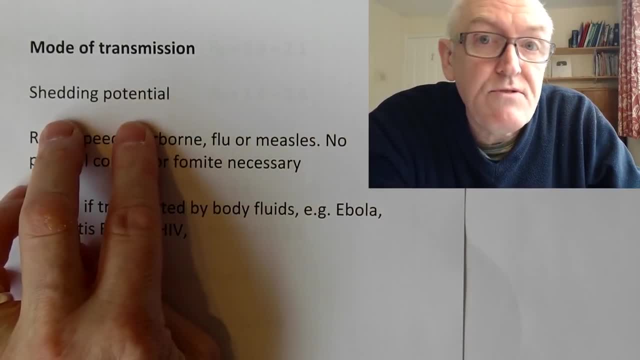 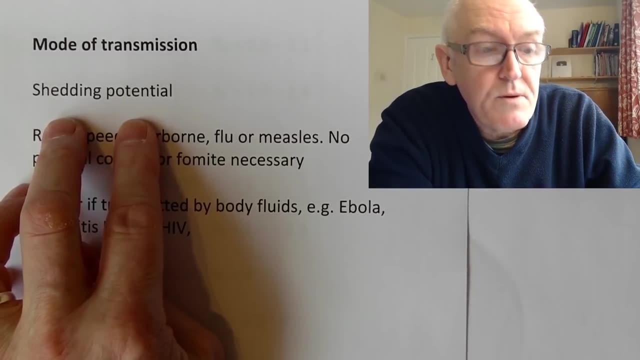 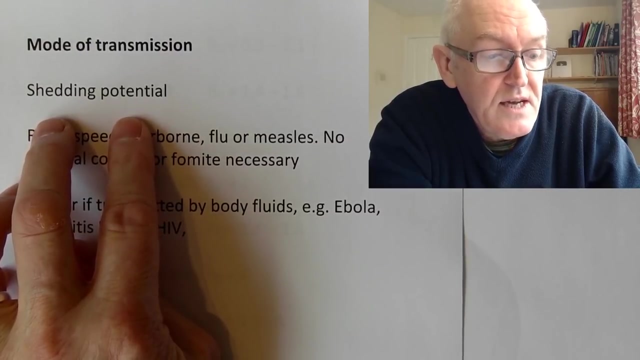 much the disease is suppressed. another good example there is tuberculosis, this bacterial infection where people can be coughing up bacteria infecting other people and again with treatment. the shedding potential goes down quite dramatically after the first two or three weeks of treatment, as the treatment starts to suppress the multiplication of the bacteria within the body of the infected. 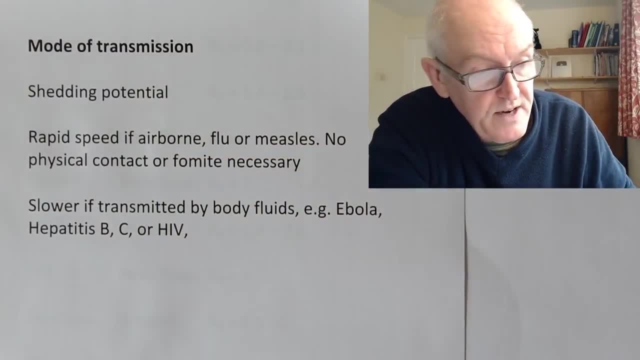 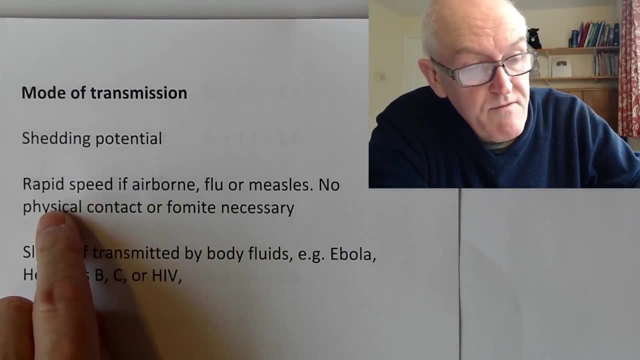 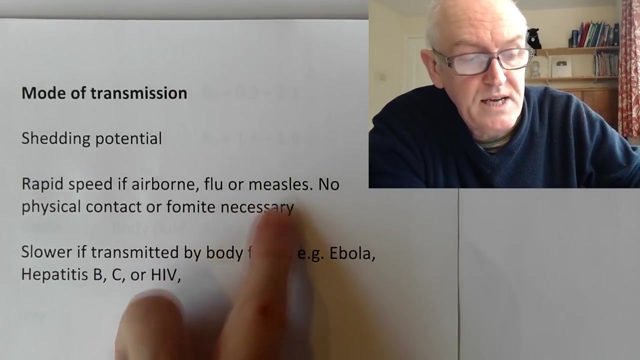 person. so the shedding potential is one important factor. now, if the virus or the bacteria is airborne, then there can be a very rapid mode of transmission. so rapid speed of airborne. so flu or measles, for example, can spread through a population very, very quickly because it's droplet and can travel in the 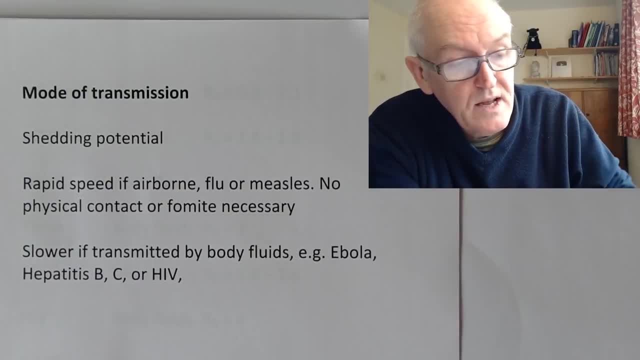 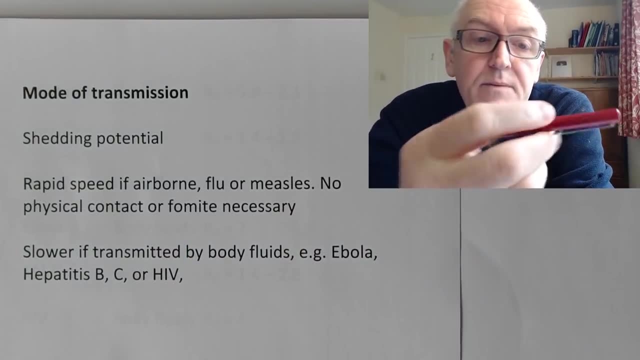 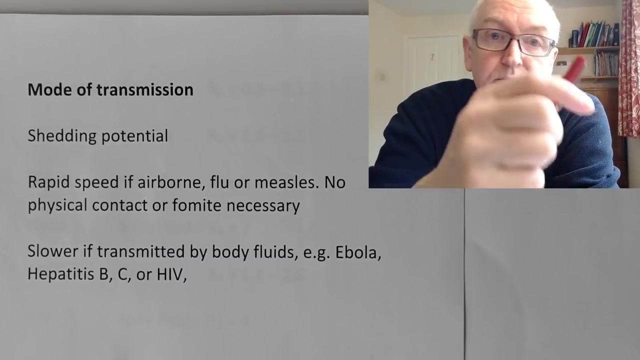 probably further in the case of measles, and no physical contact or fomite is necessary. now, a fomite is something like an object. so if I'm an infected person and I touch this pen or these days quite commonly a mobile phone, and then you as an uninfected person pick it up, 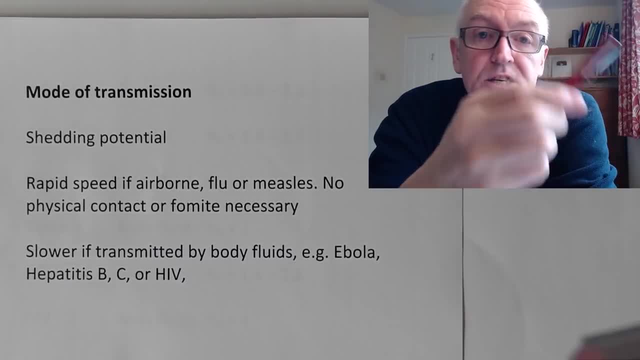 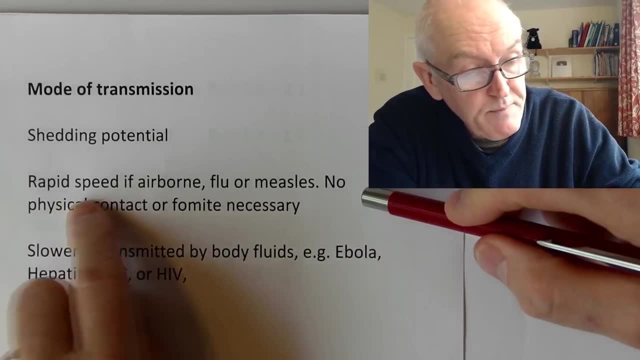 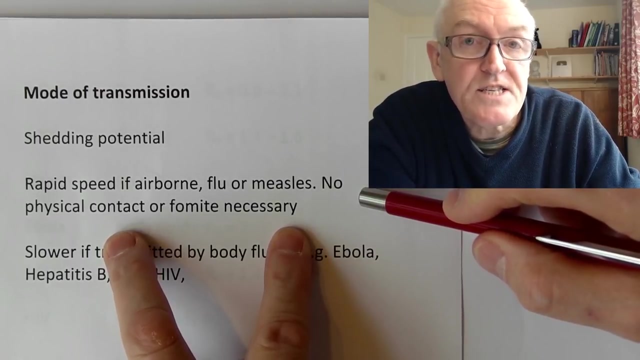 you catch the virus or the bacteria from my pen. this pen has become a fomite. so a fomite is an object which actually spreads the disease. so rapid speed of airborne flu or measles, no physical contact or fomite necessary. now these droplet infections can spread directly from person to 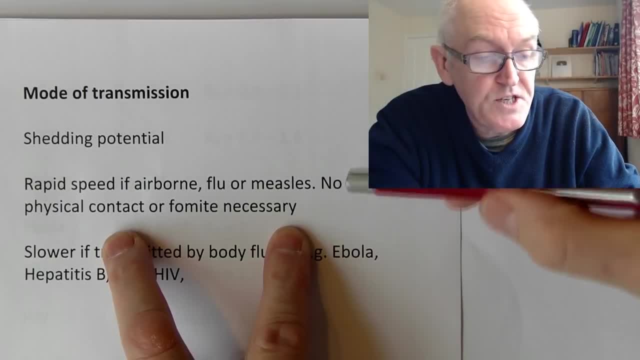 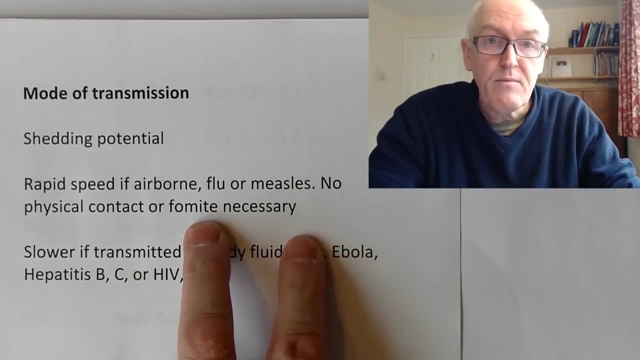 person, or they can go via a fomite, so these can actually spread via both modalities, but a fomite is not actually necessary. or a fomite could be a cash line machine where someone has coughed on and they use it and then you come and touch it with your fingers. 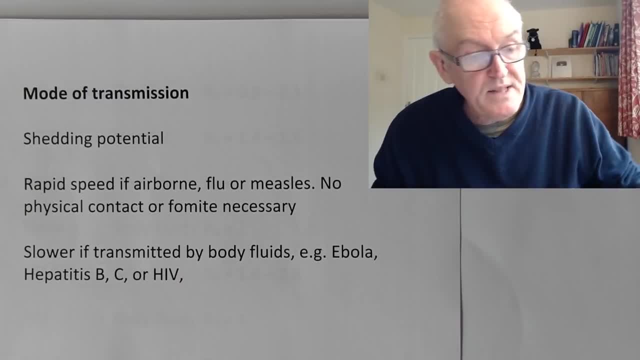 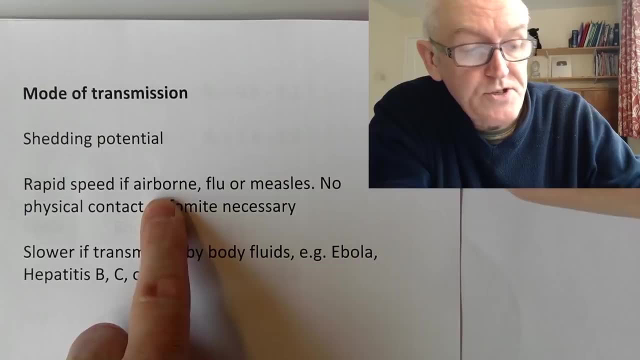 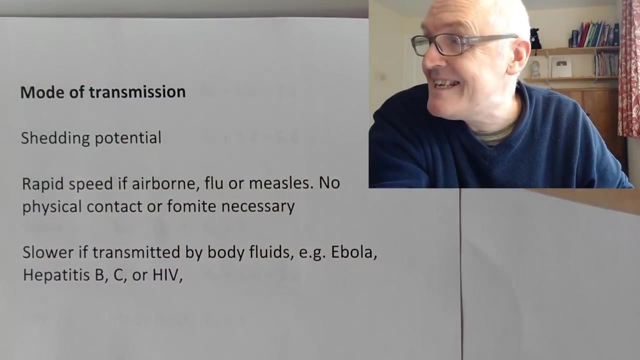 and then you contaminate yourself with that. but that's not necessarily required if it's airborne, because it can be direct from person to person in the air, but it can also be through a fomite, so that will give us a rapid mode of transmission, as people are shedding the virus into the. 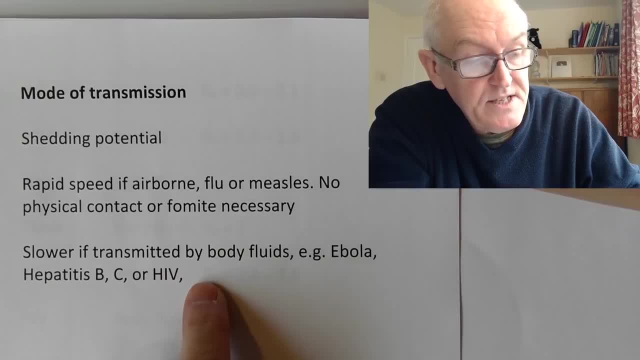 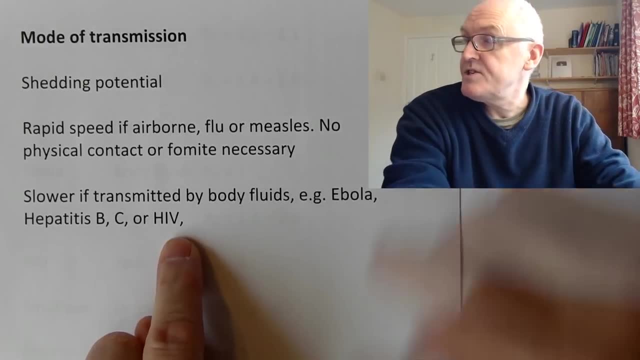 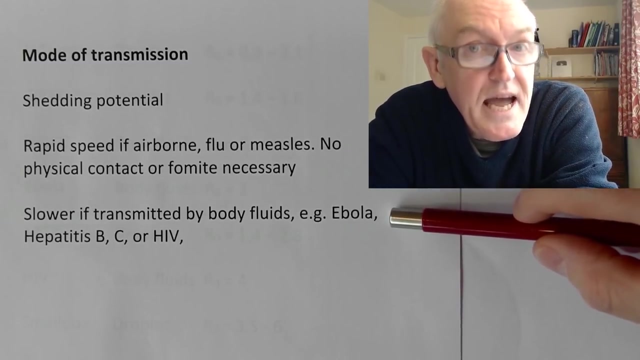 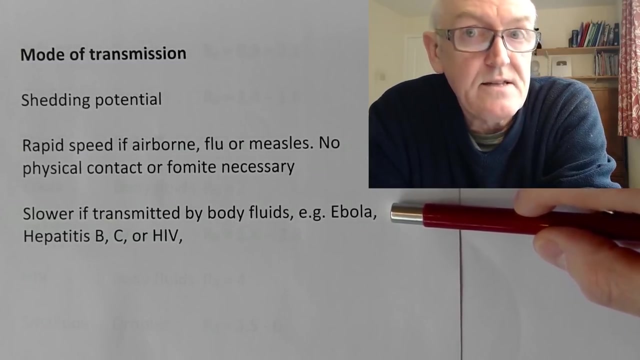 environment, but there's a slower transmission rate if it's spread by body fluids. so, for example, Ebola, hepatitis B or C human immunodeficiency virus are spread by body fluids. now in the Ebola outbreak one of the big problems was care of the dead people that died of Ebola. the funeral rites often involved infecting those that. 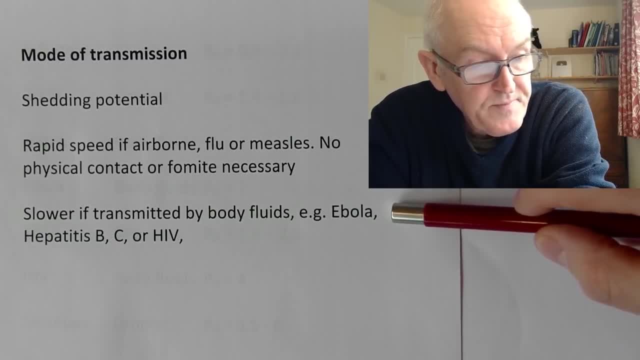 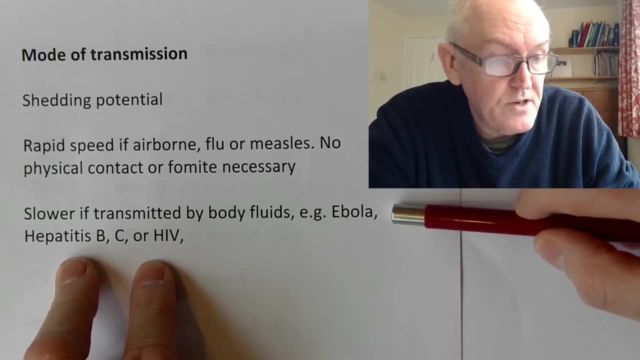 were taking care of the funeral rites and that had to be altered. but hepatitis B and C and HIV are famously sexually and serum transmitted, so they're transmitted by body fluids, so they're transmitted by cervical secretions In sperm In new bodies. So this is quite. Check the rest of this video. 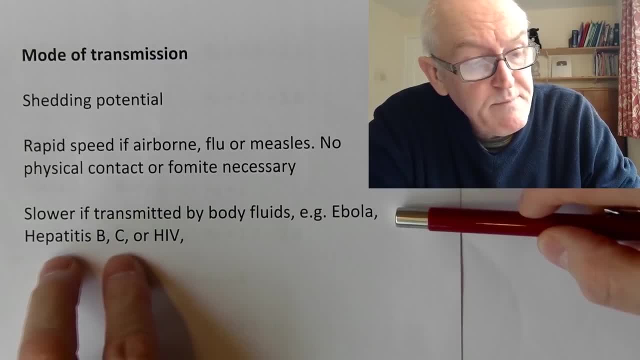 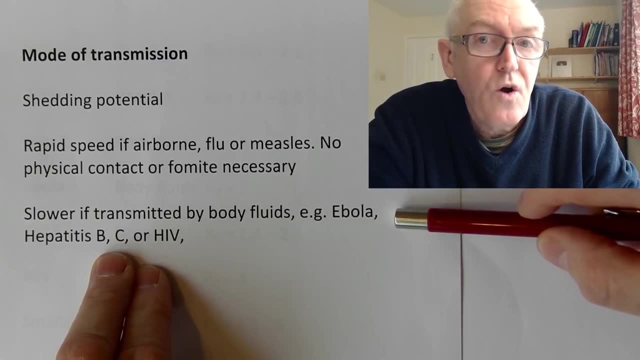 in the seminal fluid at least. And hepatitis B and C are often transmitted through sharing dirty needles amongst intravenous drug users or, appallingly, I'm sad to tell you, there are many cases where these diseases have been spread by bad quality, negligent health care. So the mode 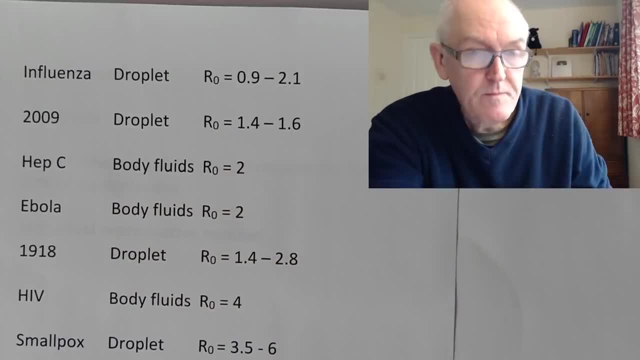 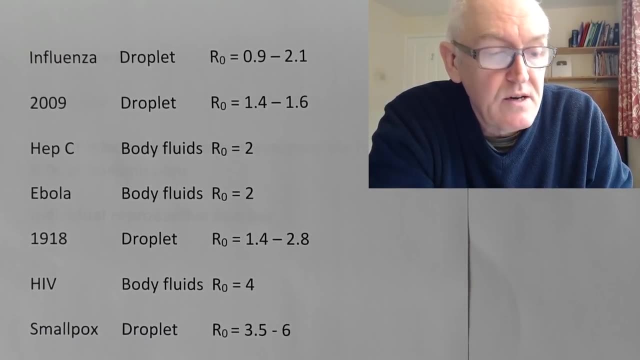 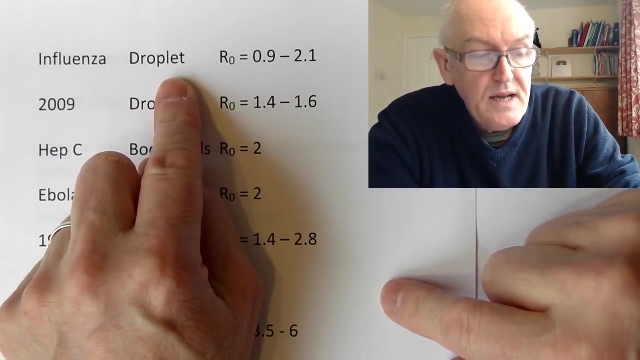 of transmission. there is going to be a big factor in the R0 as well. Let's give some concrete examples of this so we can see how this really relates to practical epidemiology and preventing the spread of infections. So seasonal influenza is a droplet infection. The virus goes into the. 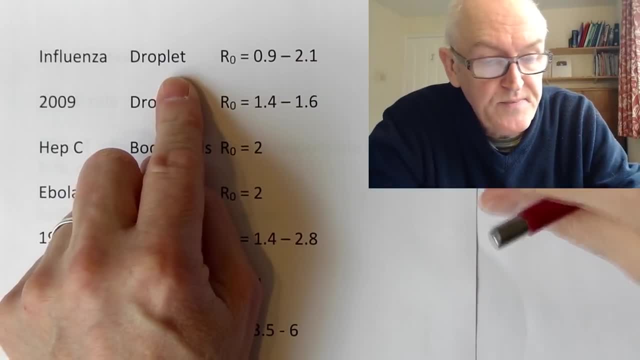 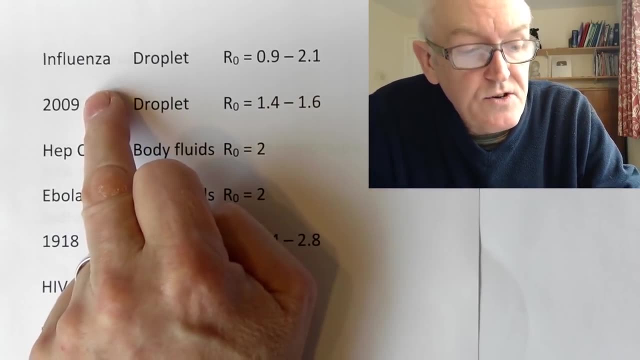 droplets that someone is breathing, coughing or sneezing out, and the R0 varies depending on the virus, because there's a slightly different version of the virus, usually influenza A, that's causing seasonal influenza, and the virus varies from year to year, So the R0 is typically nought. 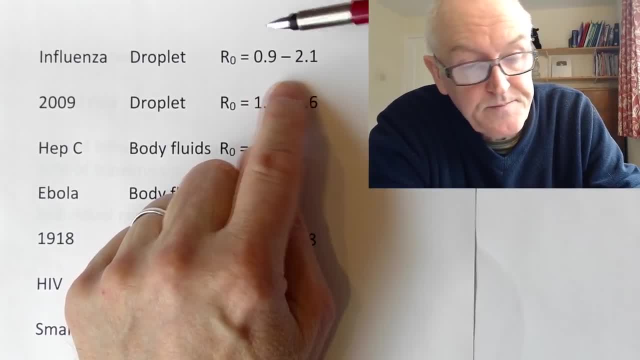 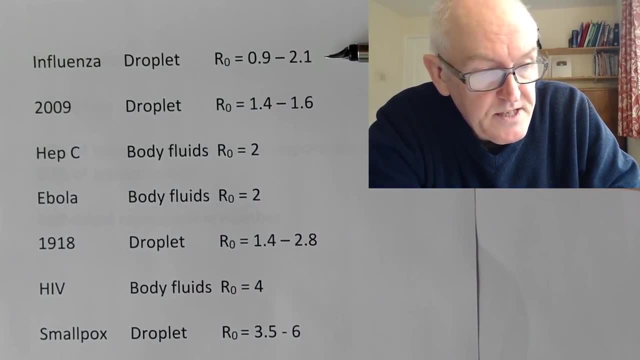 point 9, which is good, which means we have a very limited outbreak, or it can be as high as 2.1.. So sort of 1.6 is probably typical for seasonal influenza. Now the 2009 swine flu outbreak that you might. 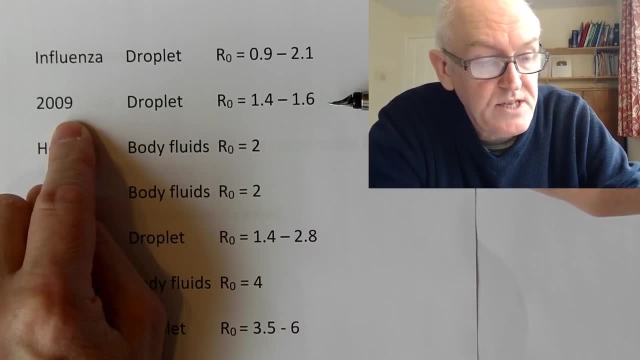 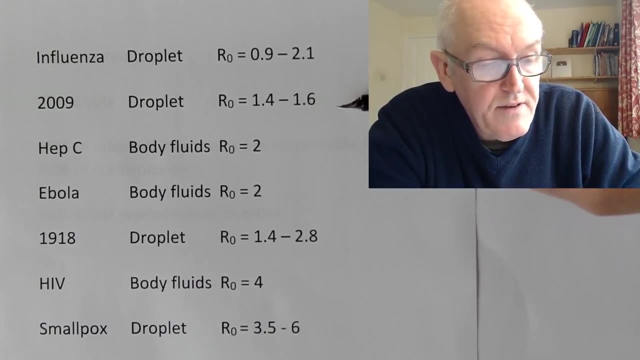 remember that was an H1N1 influenza virus. that was a droplet infection and the R0 there was in that kind of range about 1.5 people were infected on average from each infected person And this is reasonably accurate Because this was worked out after the event, where you can examine how the infection increased in. 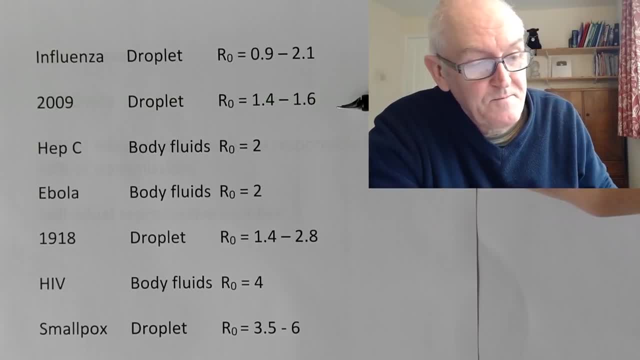 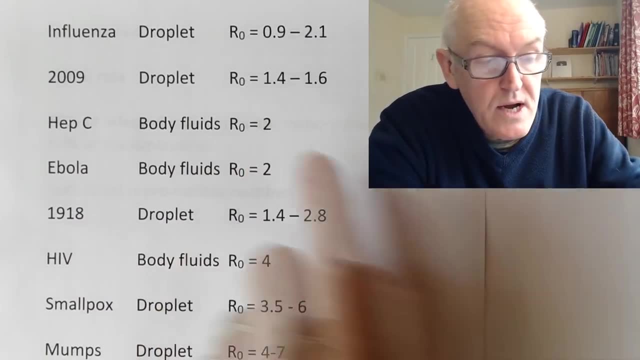 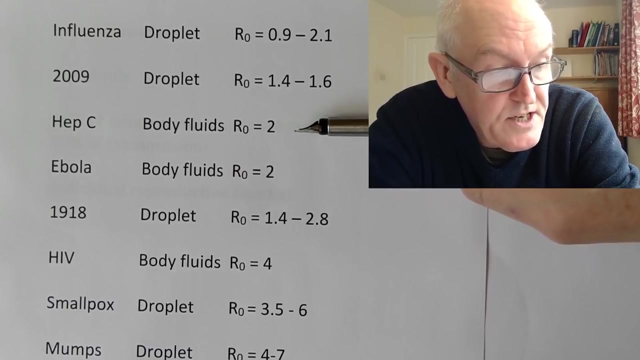 prevalence quite accurately by looking back at the data. Hepatitis C is spread in body fluids and the practical R0 there is about 2, largely because it's spread through intravenous drug users. Hepatitis B and HIV hepatitis B is probably similar, Although hepatitis B is more transmissible. 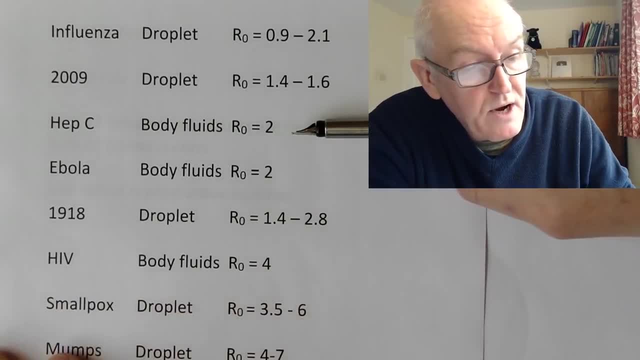 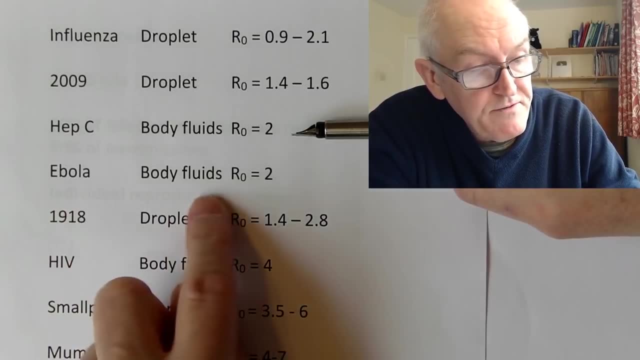 than C. Hepatitis B is probably similar, Although hepatitis B is more transmissible than C. Sometimes it's a separate topic, Right, Ebola: Hepatitis B is much more transmissible than HIV as well. Ebola body fluids: the R0 was 2.. Trouble with Ebola is the case: fatality rate was so. 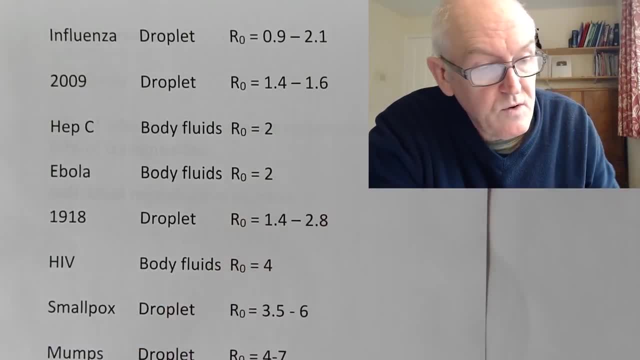 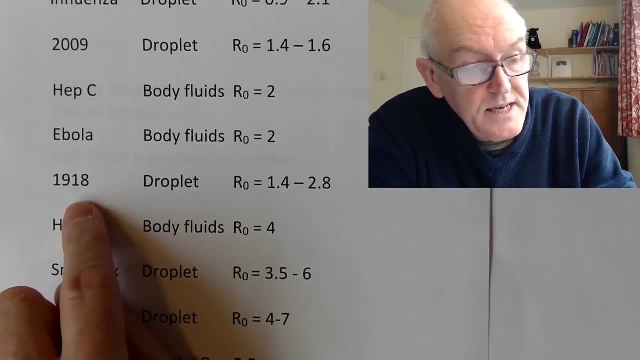 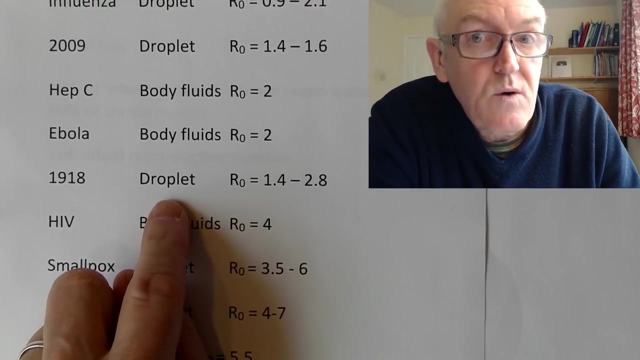 frighteningly high, So the consequences of getting that disease were really quite serious. Now the 1918 influenza pandemic- 1918-1919 influenza pandemic- spread around the world and killed 50 to 100 million people. It was a quite appalling outbreak And that was a. it was a. 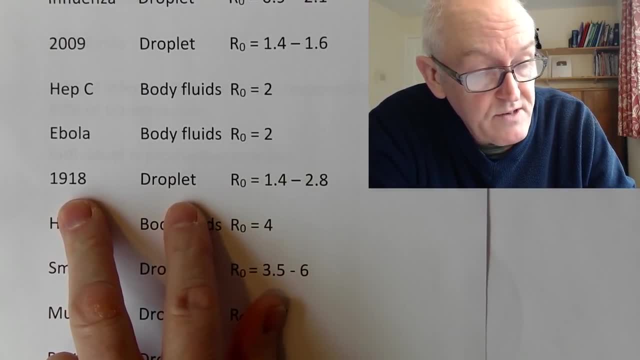 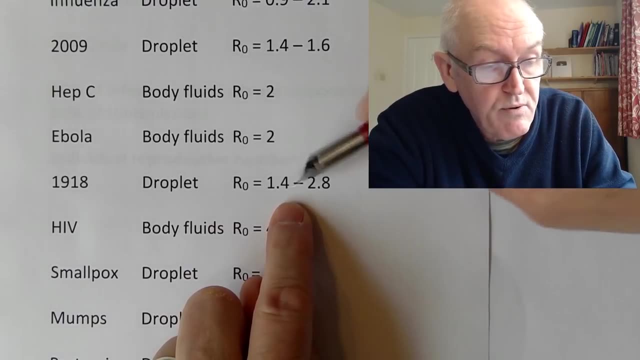 influenza A. It was an H1N1 influenza virus actually And that killed between the R0 there that the rate of spread. it killed an awful lot of people, But the rate of spread was 1.4 to 2.8.. 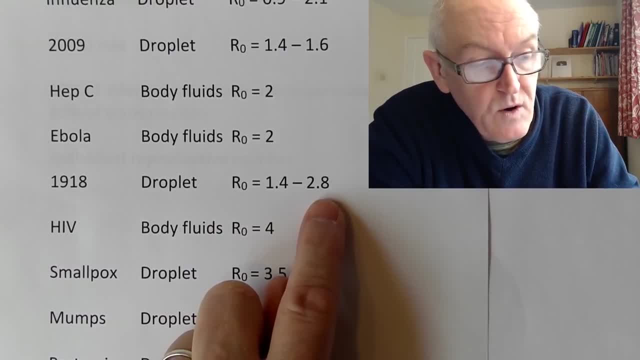 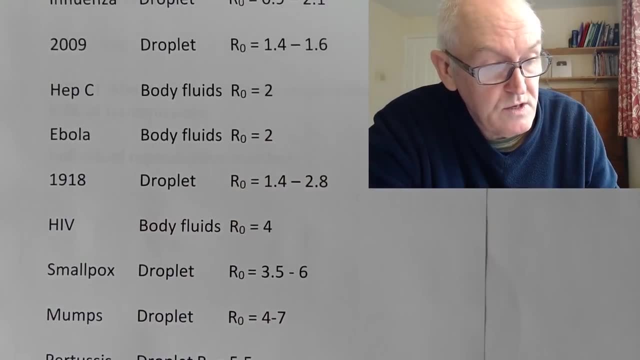 So probably figures around about 2, 2.2 are typically quoted for that. So again a high R0, partly explaining why this was a pandemic and spread around The world. HIV spreading body fluids, That's got a high R0. But that's largely because of 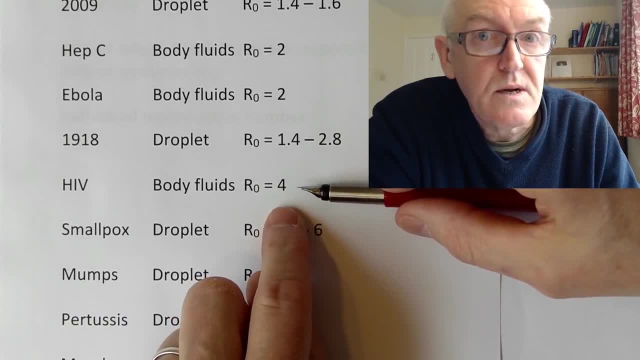 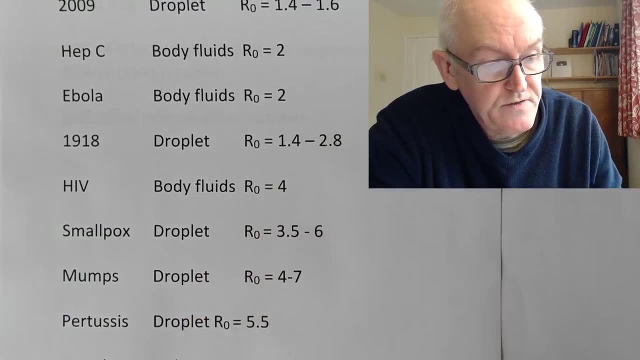 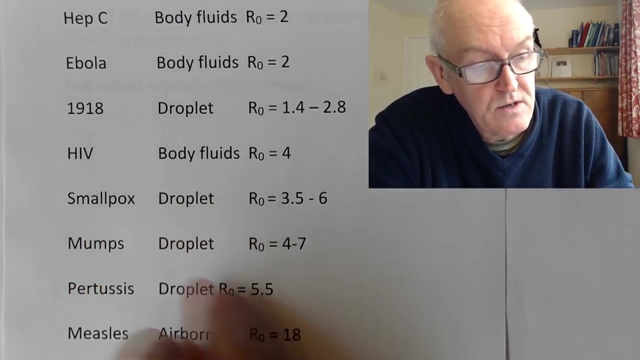 behavior, People often having multiple sexual partners, or because of people sharing multiple needles amongst intravenous drug users. Now smallpox, a wretched scourge of the past that hopefully there's now thankfully been eradicated from the world. That was a droplet infection with 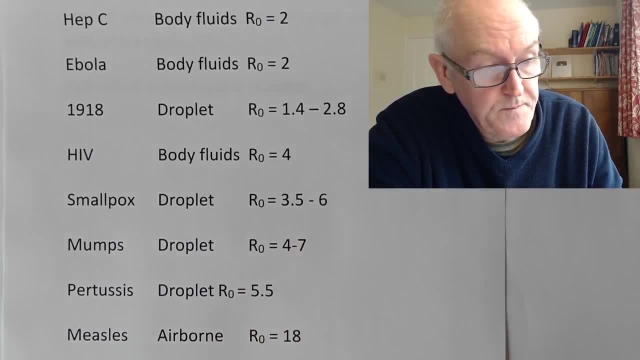 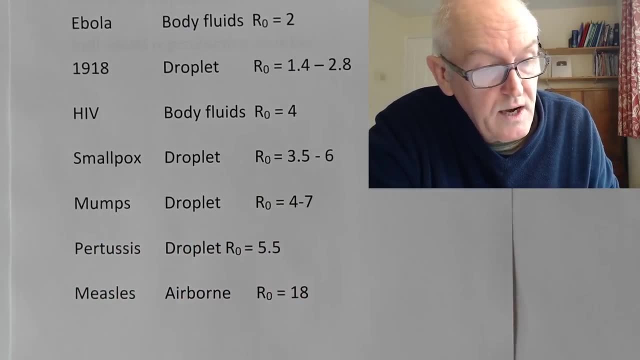 a high R0, quite a transmissible condition: Mumps which is infected, paratitis, Droplet infection, between 4 and 7 R0, so quite high. Pertussis, German measles, the R0 there is 5.5, quite high. But then one of the most infectious: 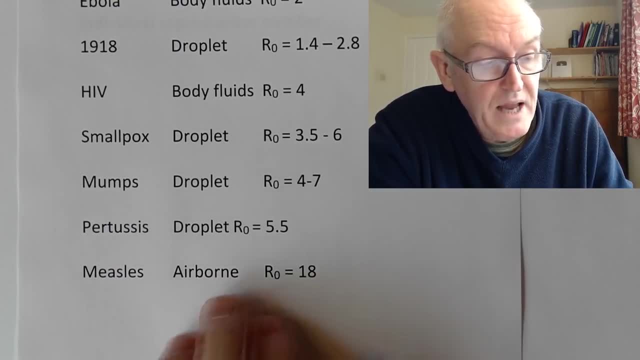 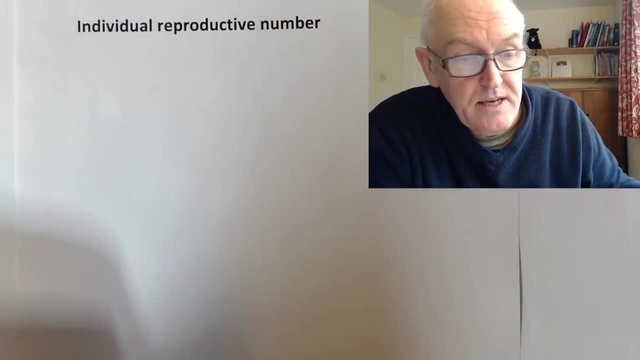 diseases around is measles, which is airborne droplet, and airborne And the R0. there can be up to 18.. Figures of 12 to 18 are typically reported there. Now, having said that, there's a phenomena called super spreaders. 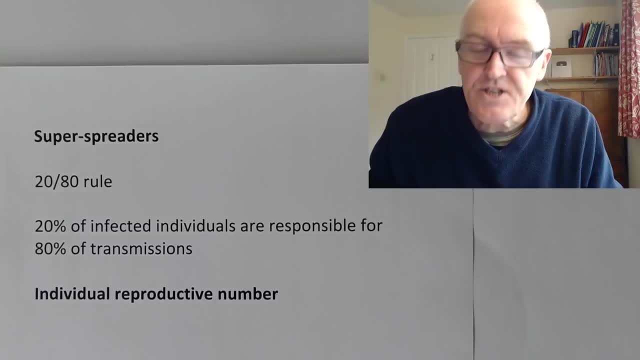 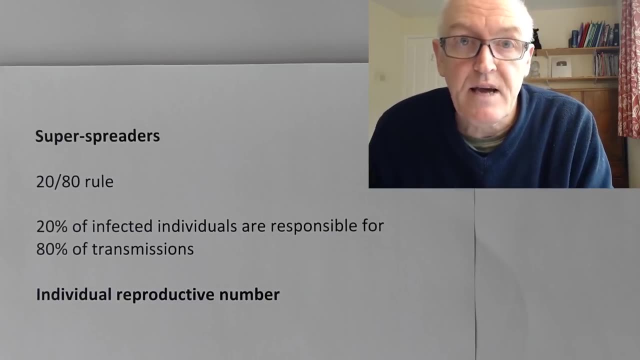 Because, remember, this R0 figure is actually an average, So really we're only going to know the R0 at the end of an outbreak, at the end of an epidemic or the end of a pandemic, looking back, looking at the growth of the infection and seeing on average how many people are infected by an 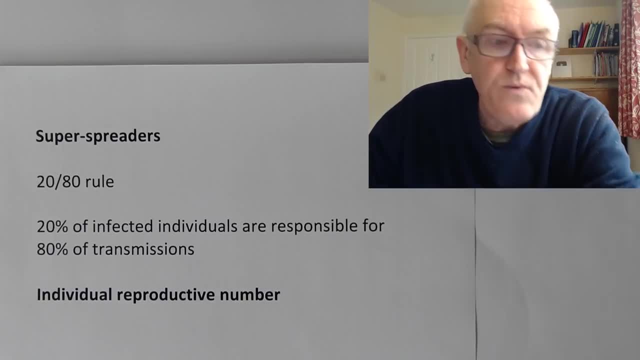 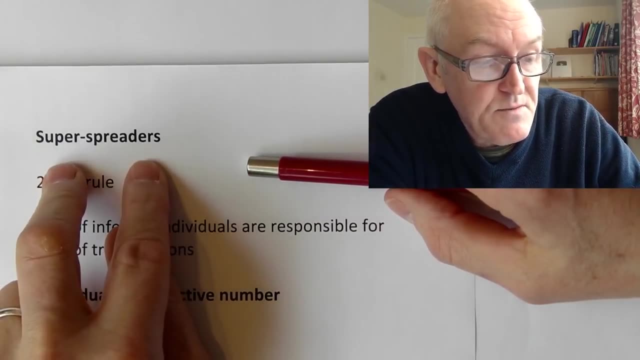 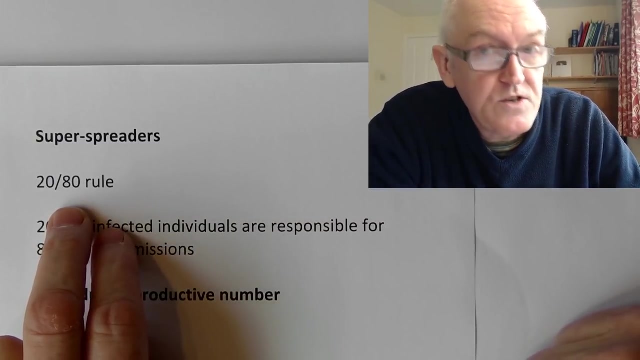 individual on average. But the way this actually works in the real world is that some people are super spreaders And I suppose you could say the converse of that is some people are mini spreaders And this is often in many pandemics and outbreaks. this has followed what we call the 20-80 rule. 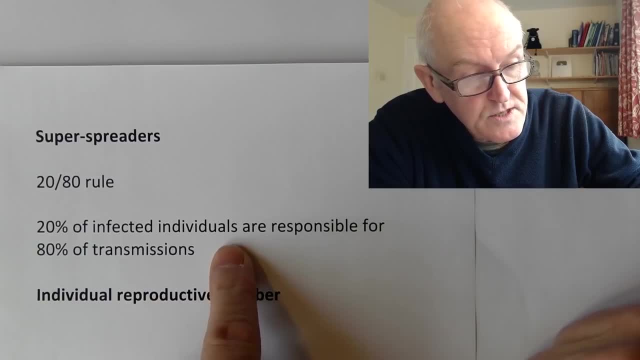 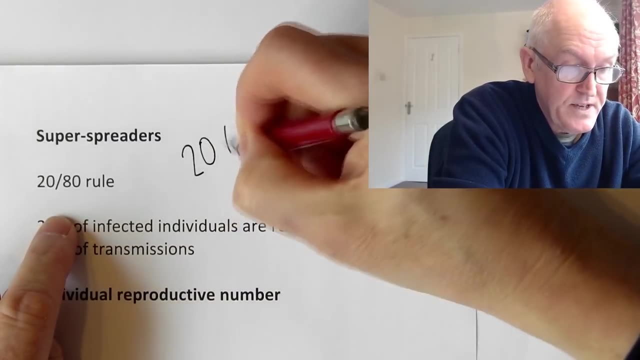 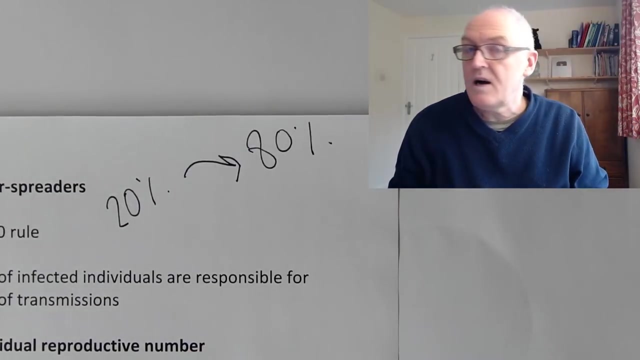 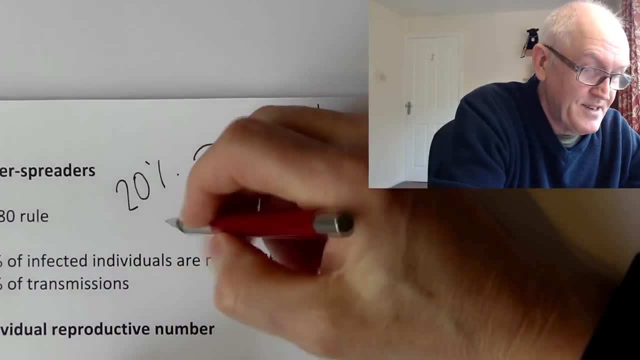 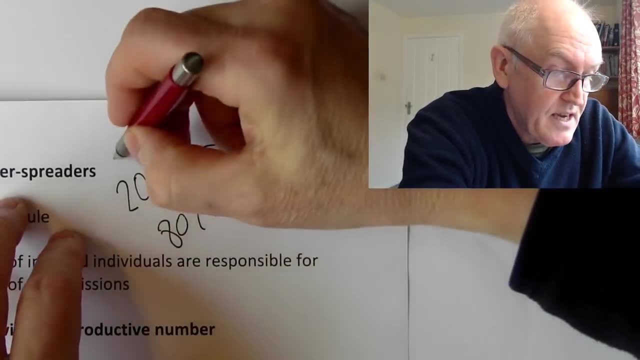 So, whereas the 80% is only infecting 20%, isn't it? So the 80% is only infecting 20% of the new cases. So the problem can be these super spreaders, And identifying these super spreaders is a big challenge for epidemiologists. 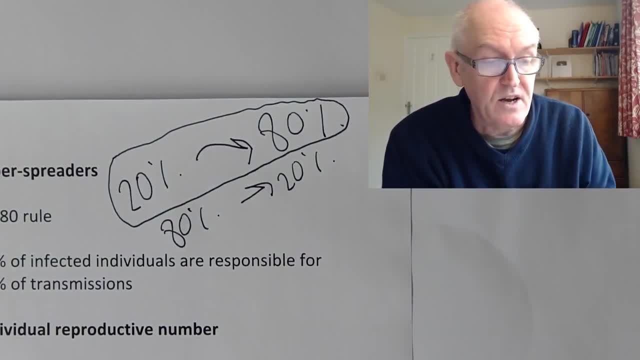 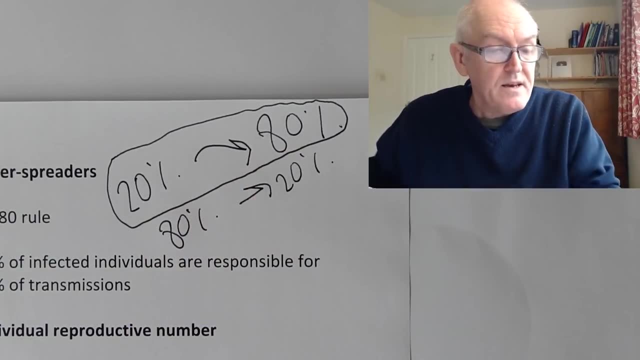 But if we cannot find them, isolate them, we're going to reduce the spread of an infectious disease, So pretty crucial that we test people to find out who these super spreaders are. Now, the biological reasons behind super spreaders is not particularly well understood. It might be partly genetics. It might be that they've had a large dose of the virus. It might be that their immune system has sort of partly combated the virus, but not enough to eradicate it, and they carry on shedding the virus for longer. 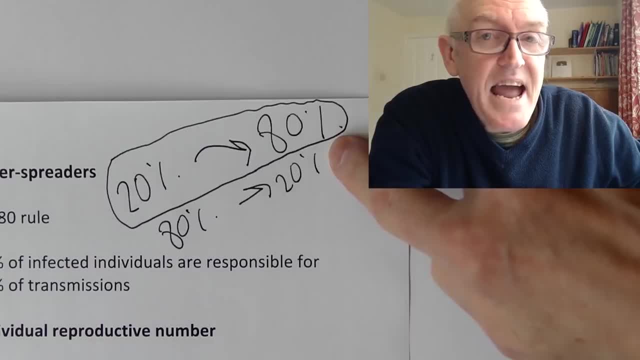 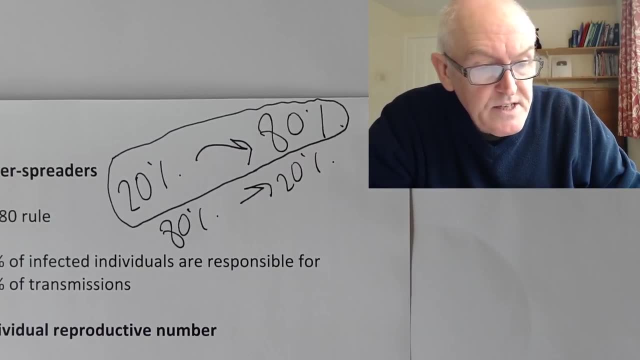 But for whatever reason, or it could be behavioural. of course, These could be very gregarious people or, in the case of HIV, these could be very sexually active people. So it depends on the nature of the virus, but this is what's often seen, that this is.